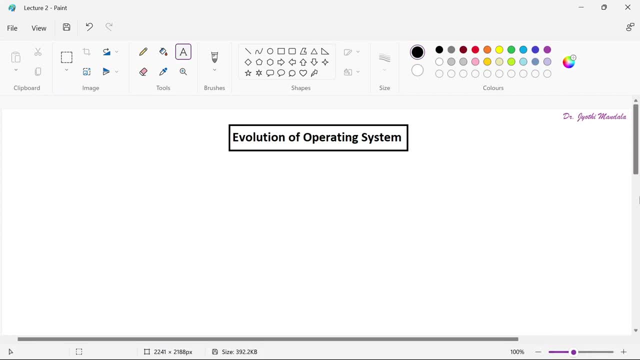 Hello everyone. myself, Dr Jyothi Mandala, Welcome you all to the video lecture series on the course operating systems. So in the last lecture we learned about the introduction to operating system. As part of that, we understood what actually an operating system is. 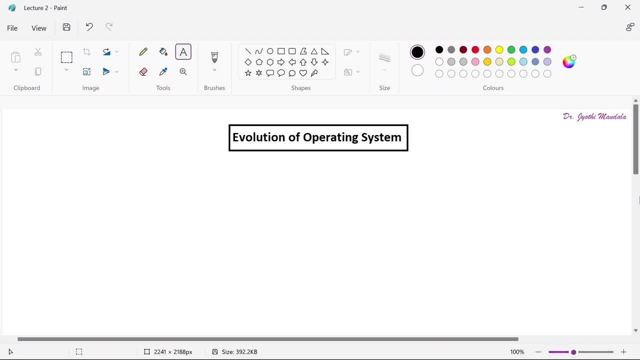 we have understood the definition of an operating system. we observed some examples of operating system. In this process we observed the difference between a system software and an application software. We understood like operating system is a system software, right. and we understood the definition. like, operating system is nothing but it is an interface between the user of a computer. 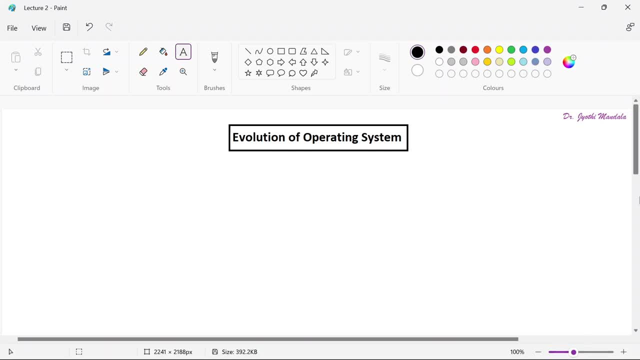 and the computer hardware. ok. And also we learned about the components of a computer and then we understood the two modes of operation, like user mode and kernel mode, which is called as a dual mode of operation, and also we understood what is timer mode of operation. 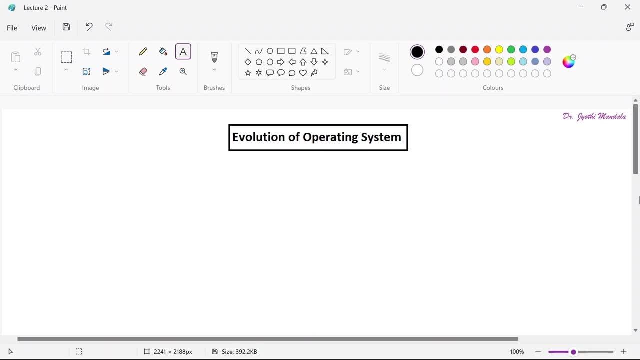 Like the switching of the operating system resources and all, and we understood what are all the services that are provided by the operating system. I hope those concepts are clear to you all. So in today's class, in this lecture, we are going to learn about evolution. 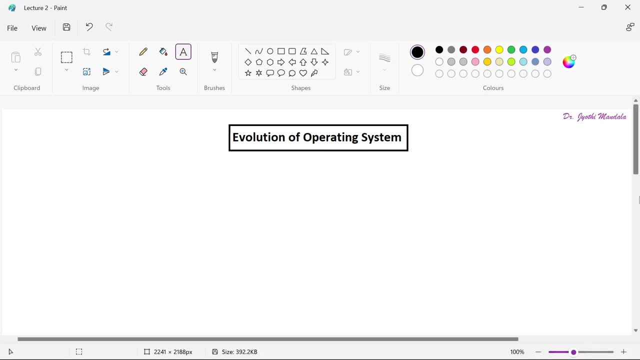 of operating system. So evolution of operating system is nothing but starting from the early systems, which is in 1950s. what sort of operating system was there in that at that time? and slowly after all, the new operating systems that are, all the different types of operating systems that. 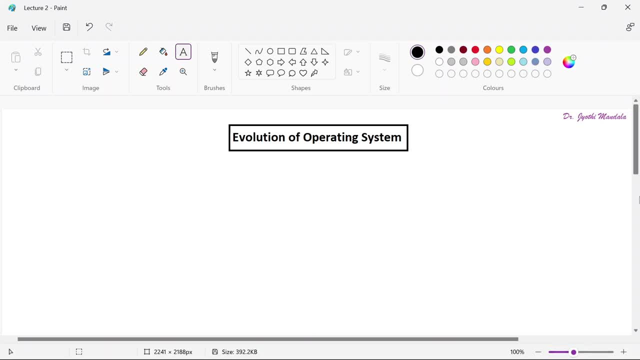 are evolved during a period of time we are going to understand. So evolution of operating system is nothing, but in turn, we are going to understand different types of operating systems. ok, So let us proceed Now. before directly learning about different types of operating systems, I want to 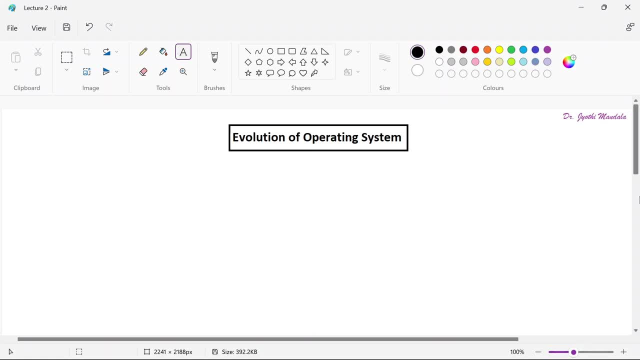 just tell, like, what is the need of, or what is the necessity of upgrading the operating systems? Can't we come with one operating system and why can't we go with the same thing? why in 1950s we have a different version and now we have a? 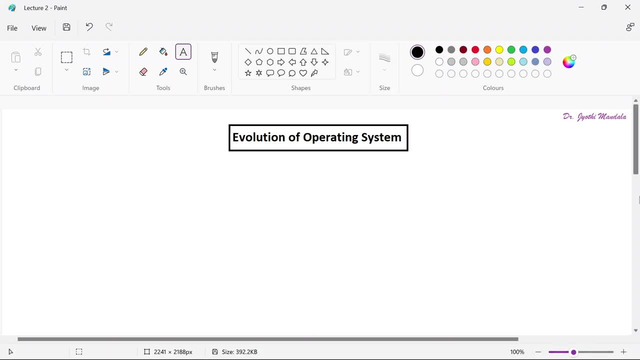 different version of operating systems. So what is the need of that one? See, operating system upgradation may be because of some things. you can make a note of that. The reasons are like we can say: there may be a requirement, service requirements may be increased. ok, So reasons. 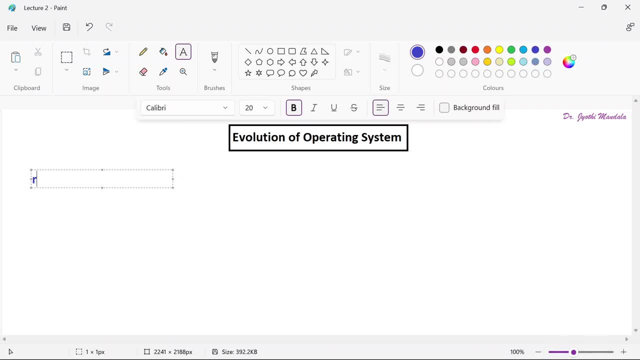 1.. Second, I just decrease the font of that. ok. Reasons for upgradation of operating system is sometimes we want to add some. what is that? a new services we want to add? ok, So if a new service is required from the user, obviously we need to upgrade our operating system. So 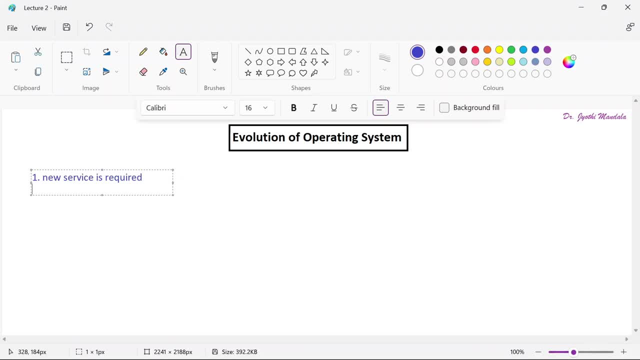 new service is required. Or else you can say an existing hardware, whatever we have, it needs to be upgraded, So existing hardware is upgraded. or else we can say: you, a new type of hardware is added. ok, In that case also, we need our operating system to be upgraded, So a new type of hardware. 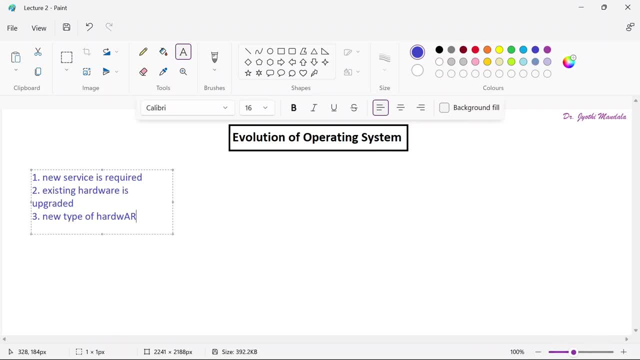 is added. that means whenever a new type of hardware is added, know to make it, the operating system is to be upgraded So that it can work with that also. ok, So a new type of hardware is added. So, considering these, some of these reasons, we can say like we need upgradation of operating system. 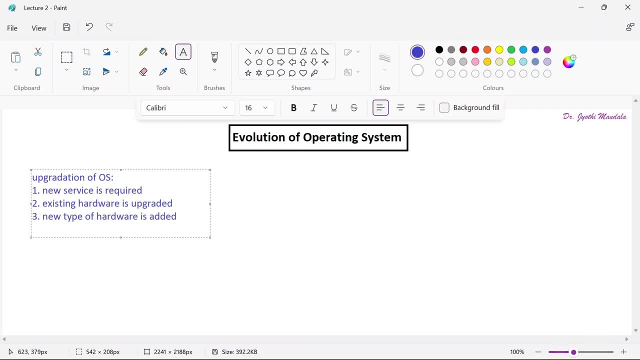 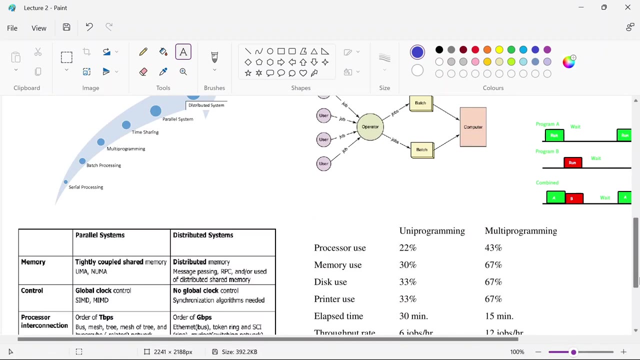 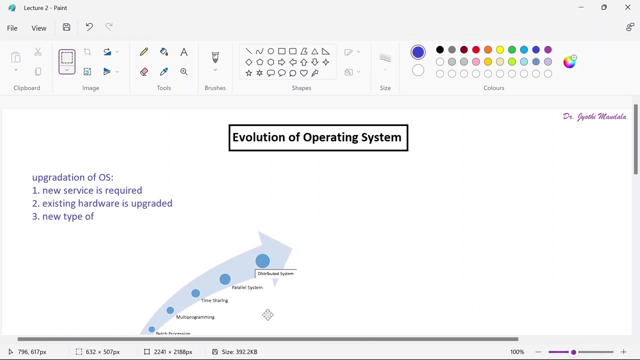 That is the reason why, time to time, the operating system Goes on upgrading. we have different types of operating system. ok, So through this, through this evaluation process, there are multiple stages of the operating system. You can see here in this diagram what are all the multiple stages of the operating system You can see. 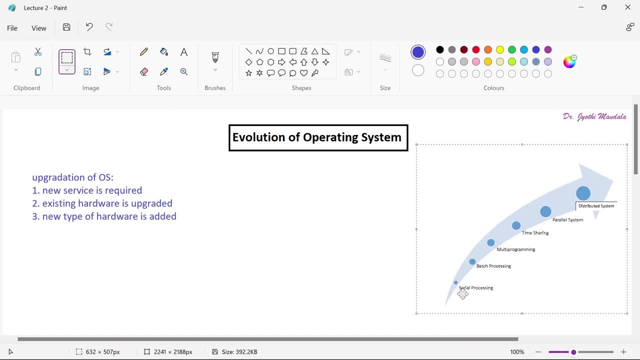 here. these are all the multiple stages of the operating system, which starts from the serial processing and then we had the batch processing, And then we had multi programming. after that time sharing parallel system, distributed system. Understand here: each and every stage of the operating system have its own advantages and 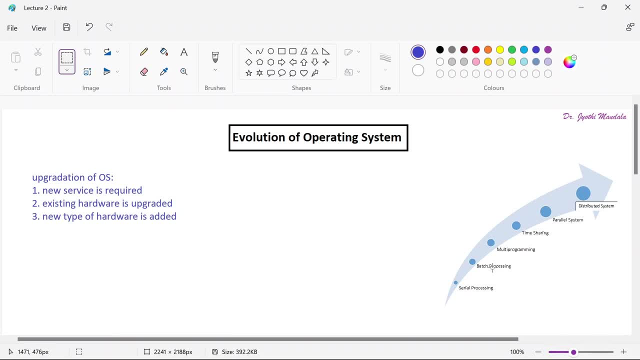 disadvantages. ok, So these can be considered as different stages of evolution of operating system, or we can also name them as different types of operating system also. ok. Now, what we will do is we will see one by one what all the different types of operating system. So let us start with. 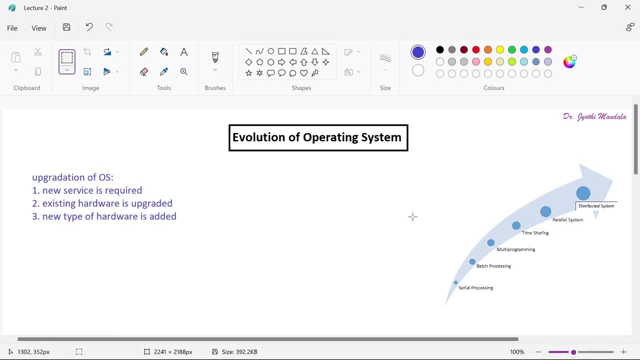 the first type of operating system, that is our serial processing. all of you keep adding that is serial processing. so the first type is serial processing. understand here it is not like only what are all reflecting here, like serial processing, batch processing, multi-programming, time, shared palette, distributed. other than this. we have personal computer systems and we can have 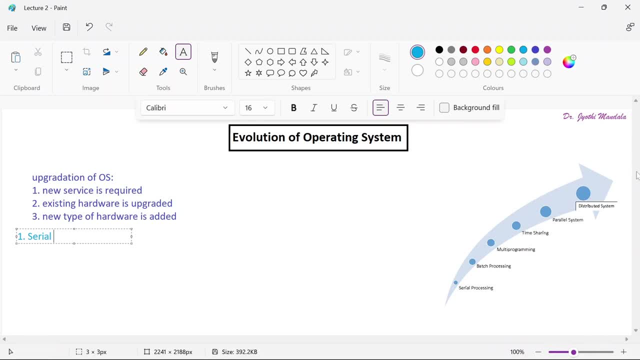 a real-time operating systems also. that also come as an evolution, and later on this we had that also- we will see that also. okay, so we will start with the first type, that is, serial processing systems. so what is this? so in this type of serial processing system, which is also called as early, 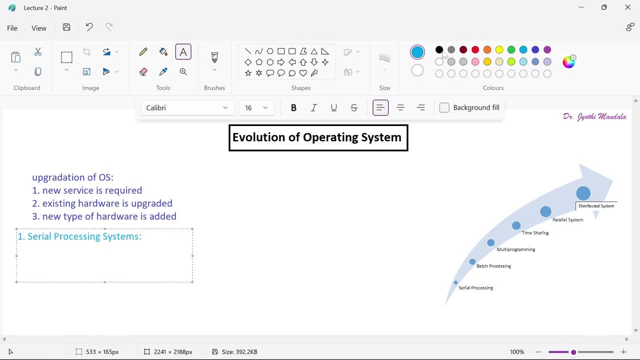 systems. okay, in this early systems, what happened is this: this is in the case like 1950s, like that. okay, so in this early systems, what happened is this: this is in the case like 1950s, like that. okay, so, these are also called as early systems. so this is around 1950s period, like that. so these 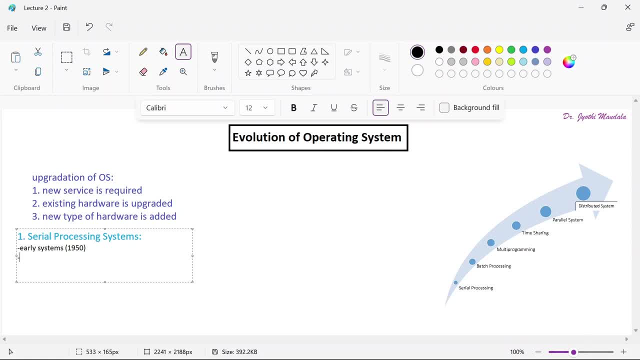 types of systems are there. now in this systems there is no operating system. there is no case of having an operating system in the early systems. now, whenever we are saying there is no operating system normally, why we use the operating system in our, in a computer? because we want to that operating. 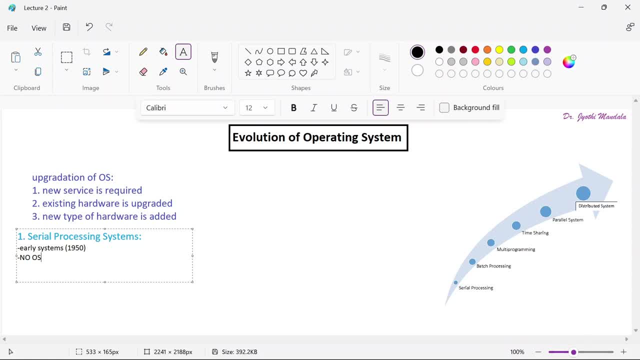 system will be acting as a mediator between the hardware of the computer and the users who want to connect with the hardware, isn't it or not? but if there is no operating system, in this case, in this first serial processing system, if there is no operating system, what is the meaning of that? 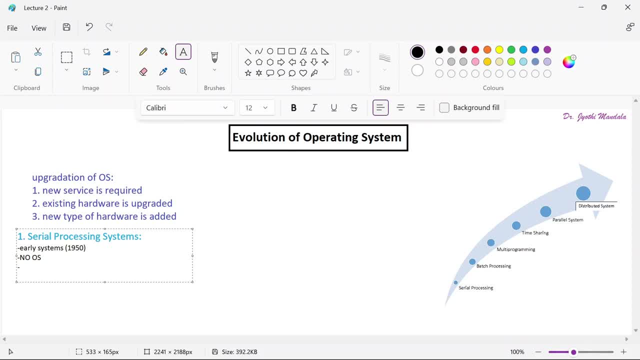 one. it will allow the programmers to directly interact with the computer hardware. so here the programmers are directly interacting with the, with hardware, because the software is operating in the hardware, because there is no operating system case. the programmers who want to communicate with the hardware, they have to directly interact with the computer. how they are going to directly? 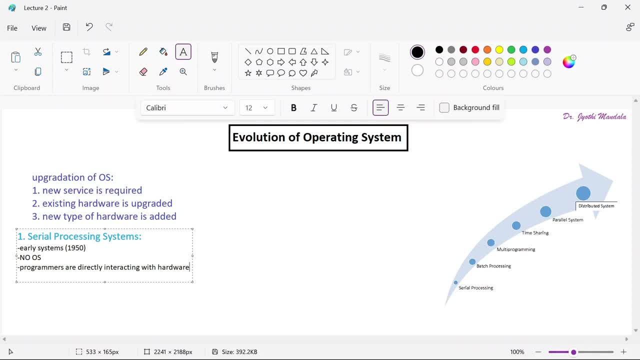 interact with the computers, like within the form of console, like they will be using switches or some input output devices, like- and they may be using some lights and all okay. now, why it is named as a serial processing system is because here, as the programmers are directly interacting. 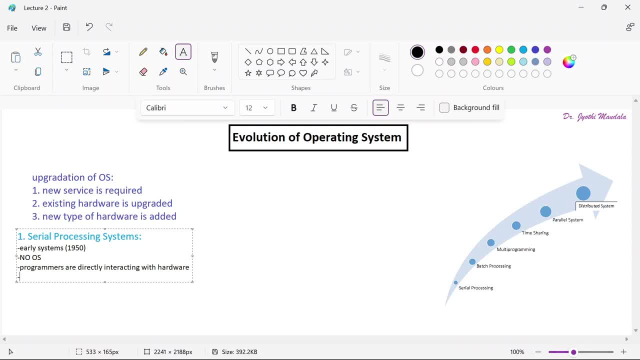 with the hardware process by process. that means once one process is done, then only another process will be considered and it will be executed. so until and unless one process is completed, another process will not be given. a chance that you need to understand here is users has to access the computer in series one after the other. that is what. so that's. 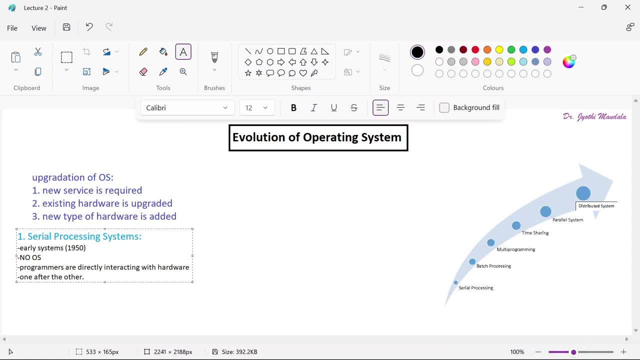 why it is named a serial processing system. got it all of you. so this is the first version where there is no operating system. in the history of 1950s there is no operating system, and because of that it see one after the other. the system has to be accessed by the users. 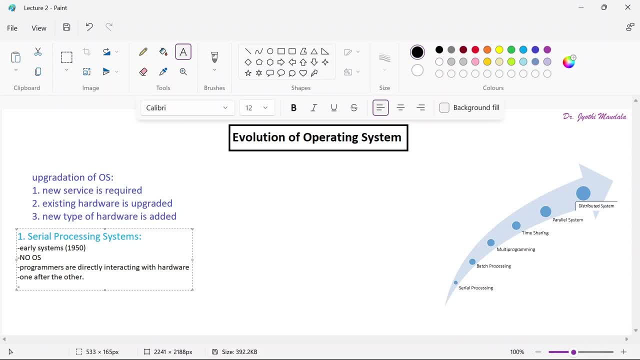 now, what is the problem with this one is it is a time consuming, isn't it or not? it takes a lot of time to perform multiple tasks. okay, so that is the thing with the serial processing. all right, i hope you all are clear with this first type of 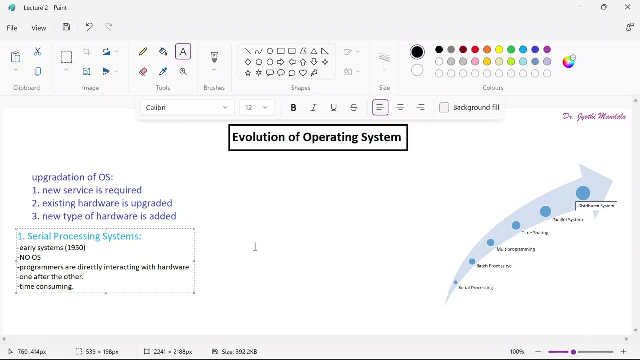 operating system, that is, serial processing operating system. all right, we'll move to the second type of operating system, that is, our batch processing. keep your heading, all of you. simple batch operating system. second type: simple batch os. now in simple batch operating system. what happens? so we in this? what happens is: 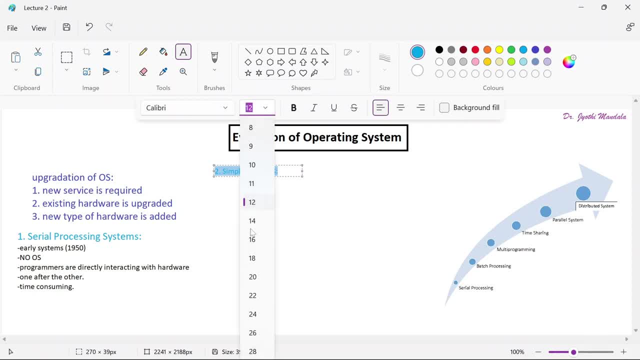 as the name itself. it is suggesting like batch. batch is nothing but, uh, a group of tasks or a group of job, in this case, process or task or anything. whatever it can be understand, it is nothing, but they will be considered as a task or process. okay, or job, all mean the same, okay. now here. 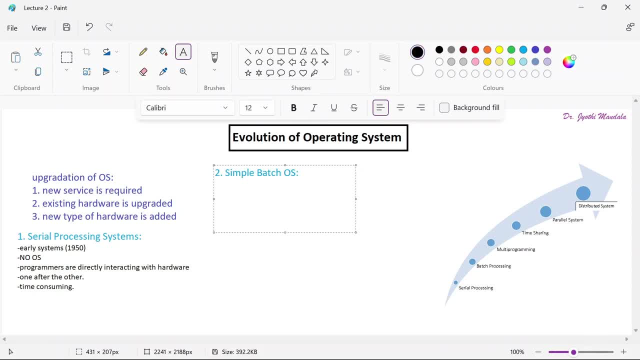 in simple batch operating system, what happens is the jobs or the tasks which are um like one second much. I'm so sorry. okay, so in this case, what happens is the tasks, like the set of jobs which are requesting for the similar needs. they are grouped together and they are formed. 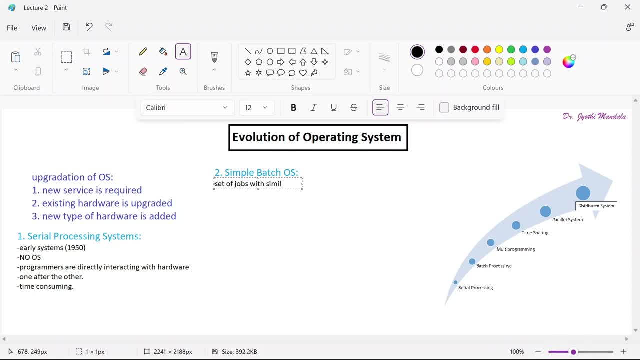 as it are, set of jobs with similar needs, are combined together to form a batch. I know the literature supports the level of gathering the workers together so that the final ritual is about that. so the units as they are å literal meaning of batch. you all know the same thing is here, but here the batch includes the. 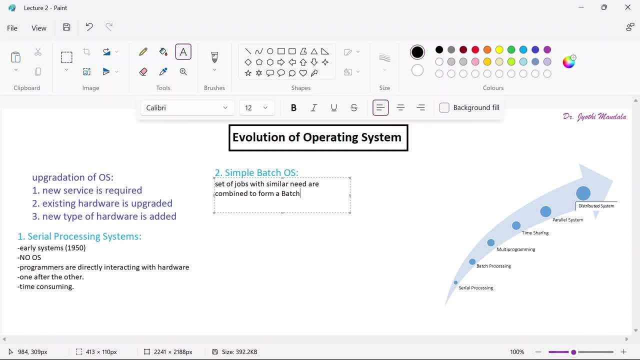 different types of jobs. where all the jobs need the similar need. they are having the similar need now. the batch of jobs will be executed by the computer. got it all of you now to understand this one here? in this concept, there is an operating system available, so there is no. 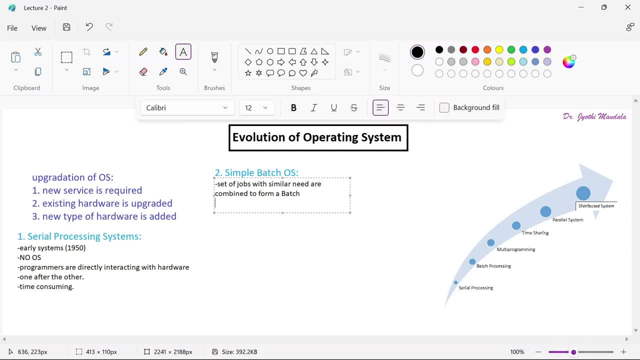 direct contact. like the, you, the. there is no direct interaction between the user and the computer hardware. okay, so in this case, no direct interaction between user and the computer hardware, or you can say computer itself, computer hardware, in this case, computer hardware got it all of you. so what is the main thing here? 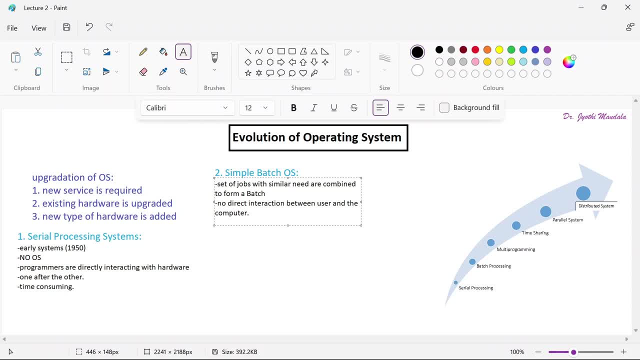 here the instructions, whatever we want to perform, the user has to give the instructions and those instructions are will be forming as a job and the similar jobs, the jobs which are of the similar needs, are combined together to form into form, into a batch and that will be forwarded to the computer. 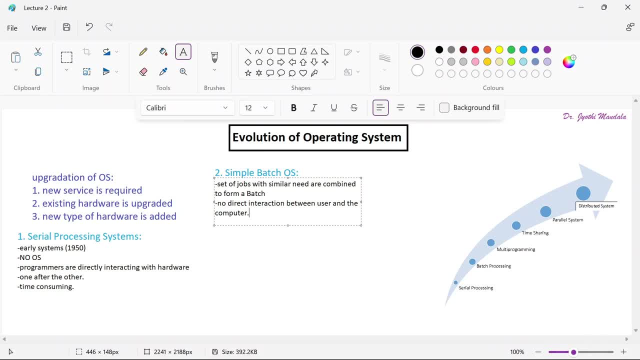 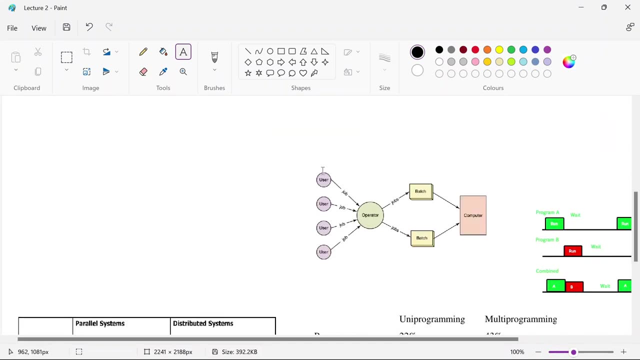 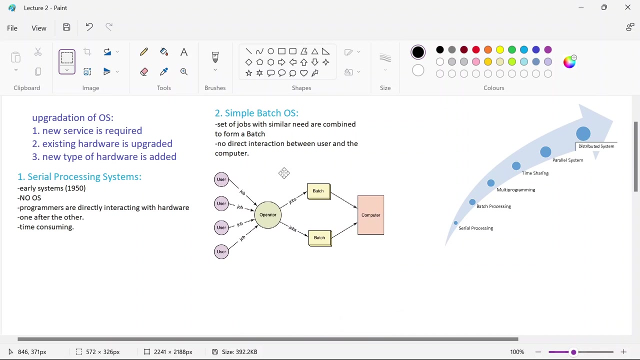 got it. so here the user will be giving the input in the form of like punch cards or in the tapes he will, the user will be giving the input to the computer. alright, so to understand this one little bit more, you can see a diagram here. you can see here what, what is happening we, that is concept for users- are they, they are giving their. 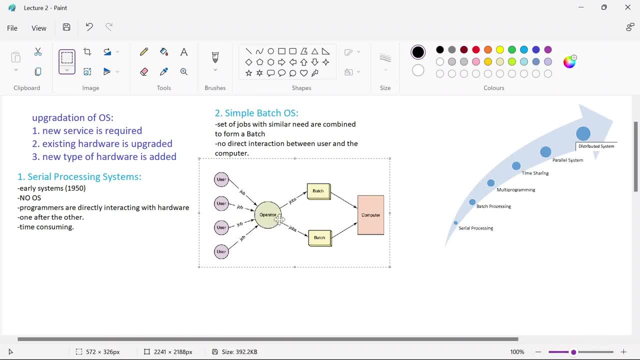 their individual jobs to a thing called an operator, who is called as a computer operator. now what the computer operator will do here. the computer operator will collect the multiple jobs from the multiple users and this computer operator will group them. will group them into batches as per the similarity of their needs. okay, now you can see here: four jobs are given and 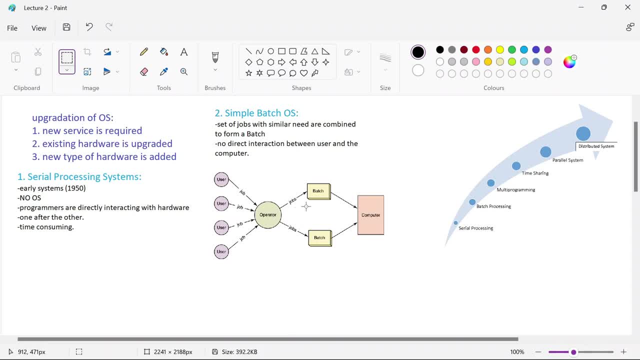 they are grouped into two batches. it cannot be two batches always. it depends upon the similarity of needs. now, considering the similarity of the need, the jobs are grouped together in the batches and then, batch wise, they will be forwarded to the computer. got it all of you here? there is a special. 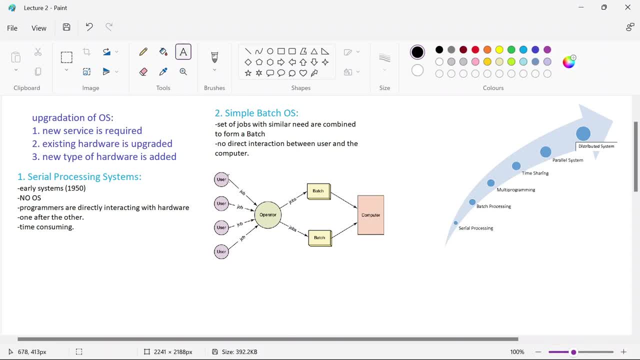 software called monitor. make a note of that one here. a special software called monitor is there and that monitor will be taking care of executing these batches, the programs inside the batches. okay, there is a monitor and monitor is a software that has to be residing in the. that has to be. 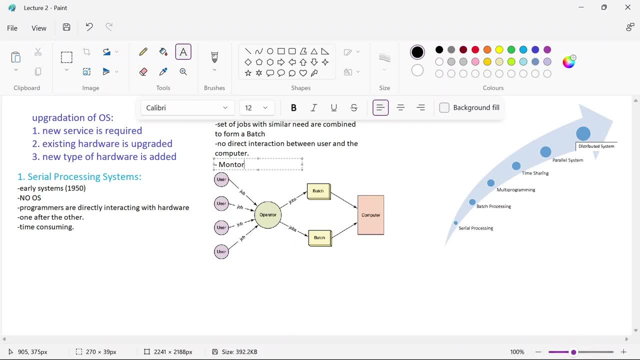 available in the main memory, because always it should be executed. okay, got it. so monitor is one software that has to be available in the main memory. and what is the requirement of having this monitor? this monitor manages the execution of each program or each job in the batch. 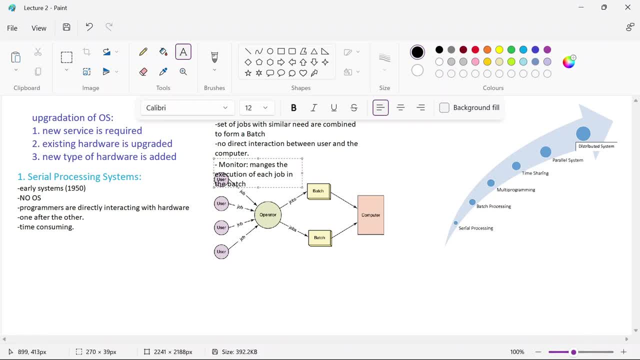 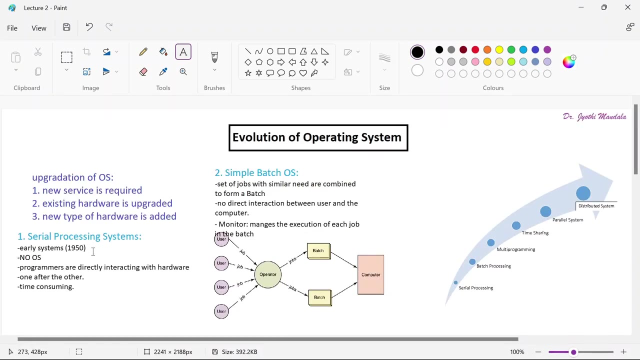 got it all of you. so this is about the monitor. all right, let us proceed further. so this is about your simple batch operating system. so, in the difference between serial processing and simple batches, here processes or jobs are grouped, put together as per their requirement, as per their needs, and then, batch wise, they will be proceeded further and 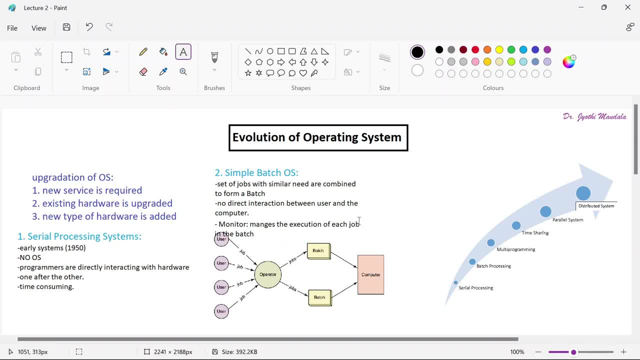 there is no involvement of, like, the user has no direct contact with the computer. you can see, in between we have a software called operating system, okay, but whereas coming to the serial processing system, there is no operating system. okay, so this is about your simple batch operating system. so now, what is the problem here is, let us 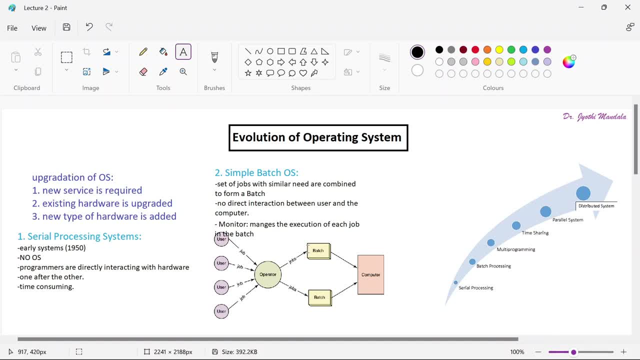 consider, one job requires i o operations to be performed, input output operations to be performed now. in that case, until and unless that batch of operations are done, it will not move to the next batch. okay, the cpu will not execute their jobs in the other patch. now let us consider one of the 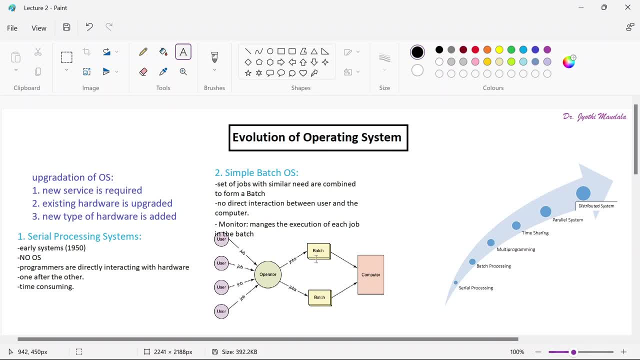 batch requires i o operations. in that case what happens? you know, it will run the actual batch. so until and unless it finishes the i o operation, cpu cannot proceed further now. at that time the cpu will be idle. that means we are wasting our processor time. processor is nothing but our cpu. 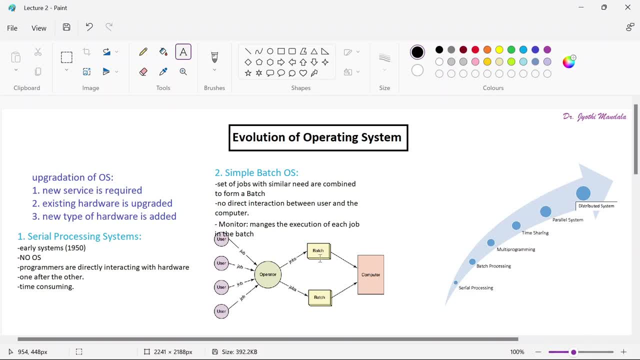 always remember we need to effectively utilize our cpu time, we need to effectively utilize our processor time. but here in the simple touch operating system we are sometimes, the cpu may be often idle. why? because because the i o operations, if it is requesting the i o operations, that speed is very low when compared to the cpu speed. in that case the cpu has to wait for that. 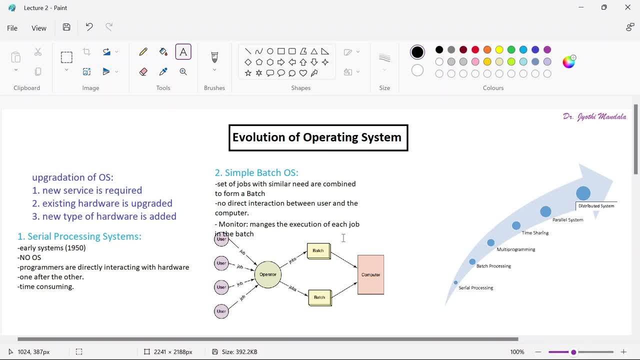 task to be completed. so that's why we can say, like the cpu may be like idle for some time, we may not be effectively utilizing this cpu time. all right, so that problem is solved in the next level, that is, your multi-programming, multi-programming operating system. okay, we'll see about that now. multi-program, multi-programming. 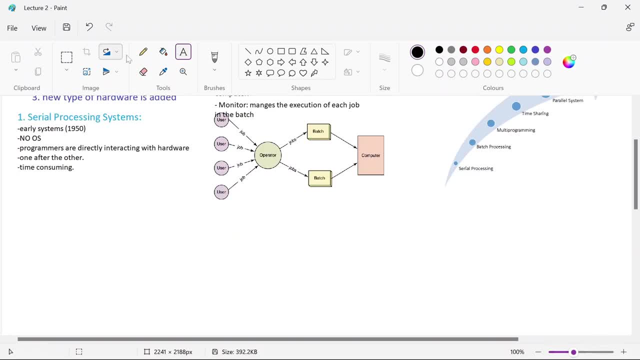 batch operating system. keep hearing all of you: multi-programming batch operating system. this is the third type, multi-programming batch operating system. now, in this multi-programming batch operating system, what happens? so, whatever the disadvantage we have observed in the this category, what is that in the first, second category of batch processing? 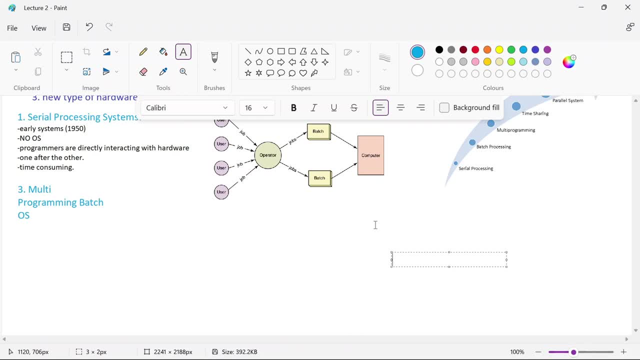 what? that we are not effectively utilizing the cpu time. so that problem is solved in this one. now, what happens here is multiple programs are kept in the memory, okay, and all are executed simultaneously. it is not like it. the processor will be waiting for one, one task to be completed. suppose you have two processes: p1, p2. 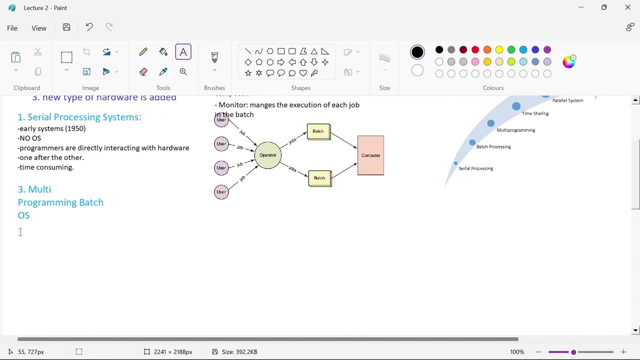 okay, just we'll see that. now let us consider we have two processes, p1 and p2. now, p1 if it is requesting for an input output work to be done. in that case, in the second option of batch processing, the cpu will be idle in that case. but here what happens is that we have to implement the massлю. 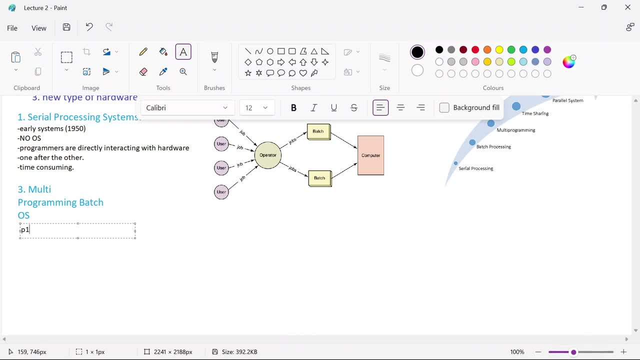 but here what happens is that the masslio is sacrifice, the cpu time, that is, state Hotel, is put in thatником the issobacker is produced after extra time, that is, the cpu will work in this software. Suppose P1 is requesting some IWO operation, okay, 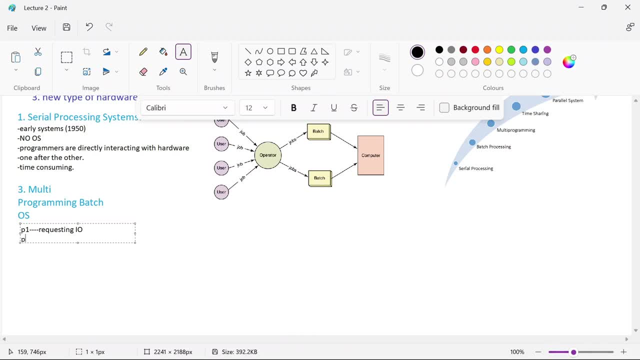 In that case, the CPU will not be idle. It will be assigned to another process Where that CPU time will be utilized to execute the sum task of our program 2 or process 2 Got it? That means we are not wasting our CPU time Instead of keeping the CPU idle. 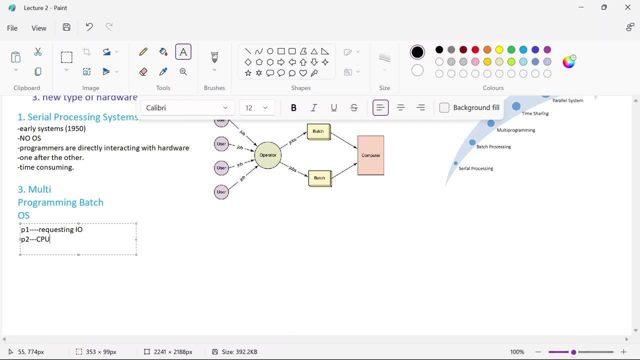 We are allocating some another task to the CPU, Got it. That means we are effectively utilizing our CPU time, Got it? In this case, the CPU will never be kept idle. That means we can understand: here is Multiple programs are executed simultaneously So that we can effectively utilize our CPU time. 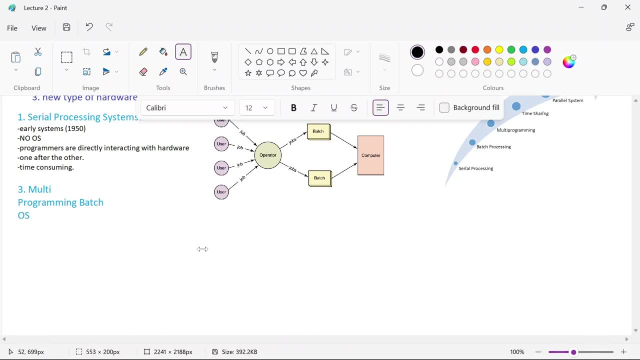 If you are not executing simultaneously, What happens? And the same thing which happened in the batch process? We may be wasting our CPU time. Okay, So effective CPU utilization is there here. Got it Now here. you need to understand the difference between Uniprogramming and multiprogramming. 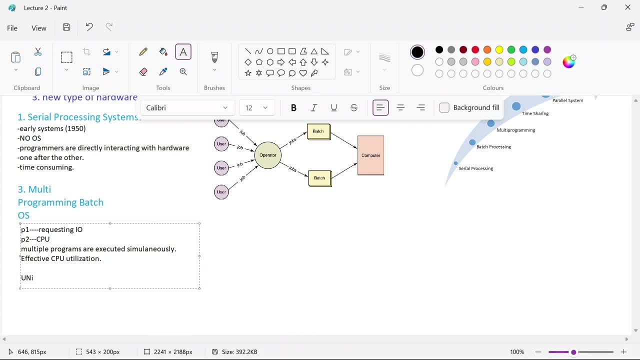 Uniprogramming is nothing, but You are executing only one task. Okay, And we have multiprogramming- Multiprogramming. What is the difference between these two? Let me highlight all those things. Uniprogramming is nothing, but we are executing one task at one time. 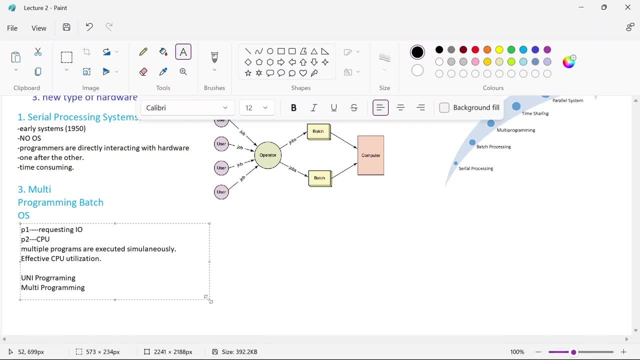 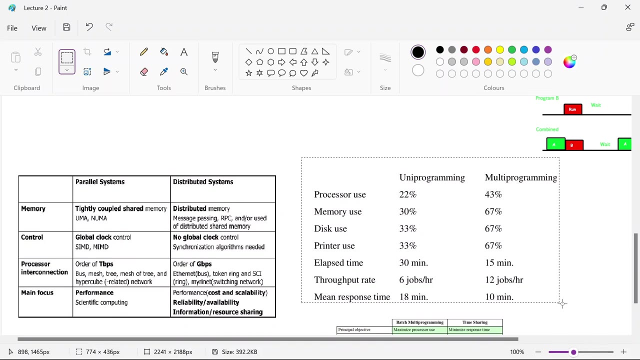 Multiprogramming is nothing but we are giving. We are not wasting the CPU time, We are executing multiple tasks at a simultaneously. Okay, So here I will highlight you the differences between The uniprogramming and multiprogramming You can see here. Okay, So here I will highlight you the differences between the uniprogramming and multiprogramming. 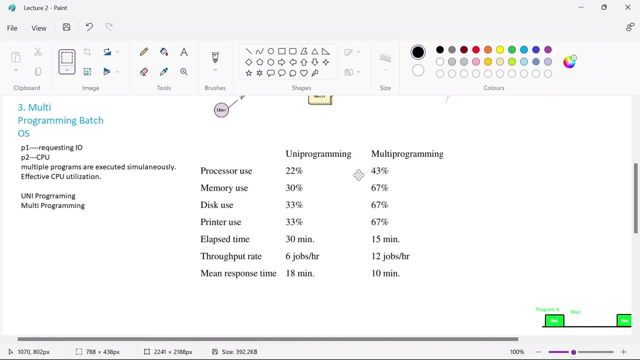 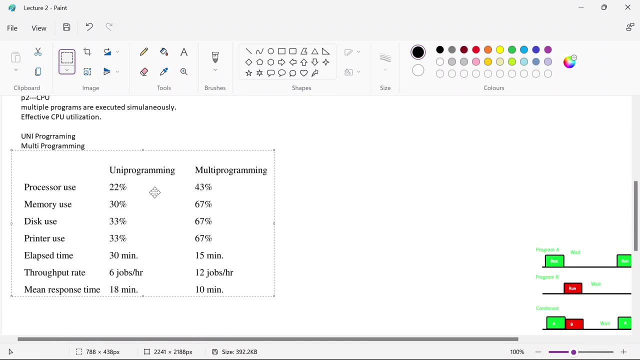 You can see here. Okay, So what are all the differences between the uniprogramming and multiprogramming is Processor use. If you see, It is understood like 22% of processors usage is there, But whereas if you are using multiprogramming, The processor use is doubled. 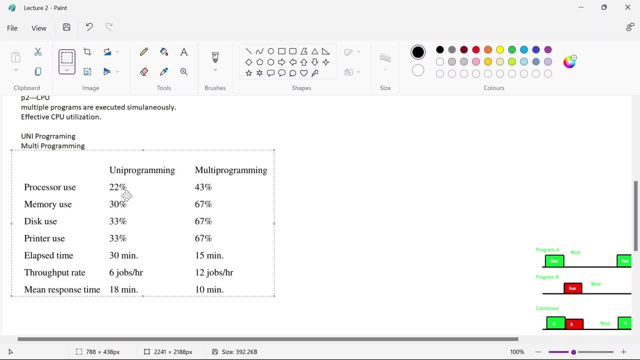 You can see Why? because Here you are executing only one program at one time, But whereas coming to here you are executing multiprograms. Okay, To understand this one, Let us take one more example. You see here what happens. Let us consider one program. Okay, Program A you want to execute. 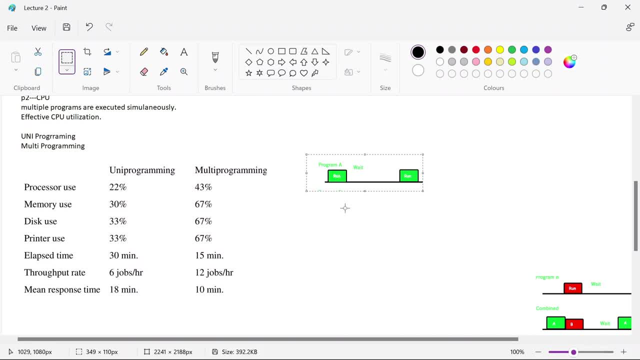 Now the program A Wherever there is run, No, it is nothing, but it is using the CPU time And it is executing that. And CPU is executing that Now after some time. it requires wait. CPU requires wait. Why? because The program A want to perform some input output operations. 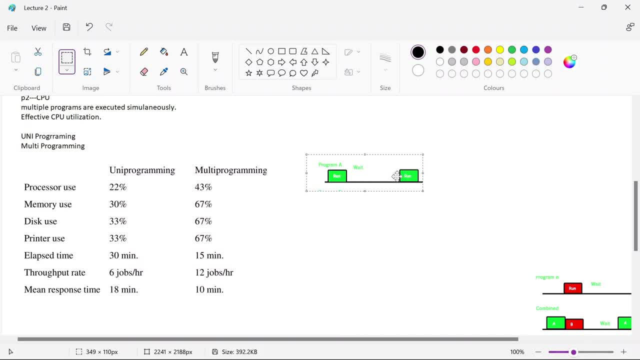 During that time, what happens? The CPU is idle. So throughout this process, From here to here, The CPU is idle. So the CPU is idle Now. after that, We will be executing this Program. A, the CPU got the chance And it is executing this program. Understood all of you. 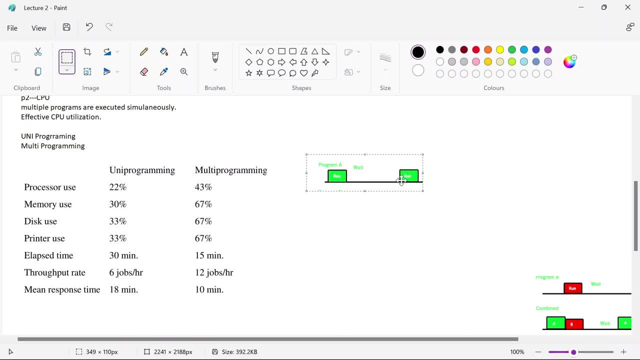 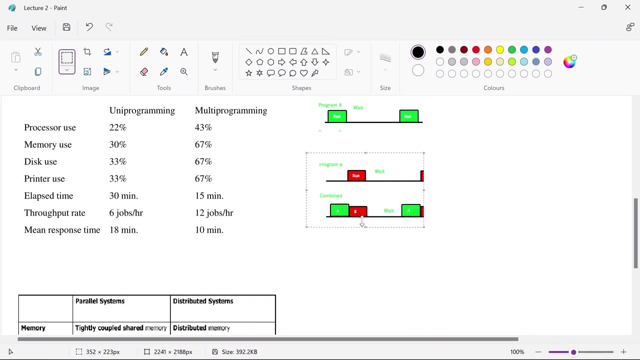 That means this time, From here to here, we are wasting our CPU time, But that is called as uniprogramming. Okay, That is what- 22% of processor only- we are using. But suppose if you are converting that to multiprogramming, You can see here. 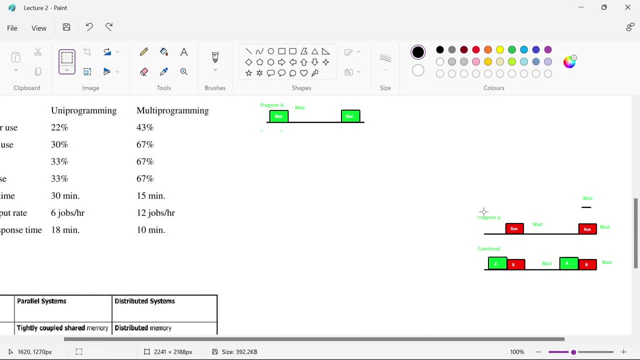 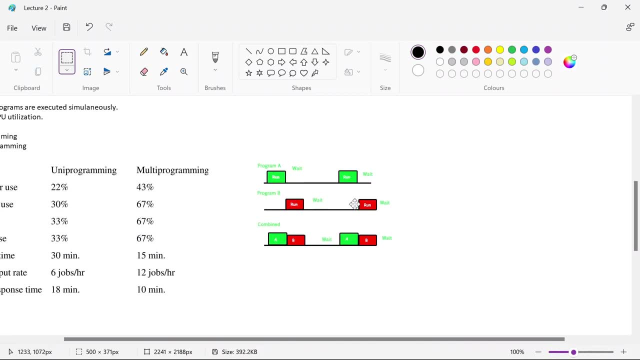 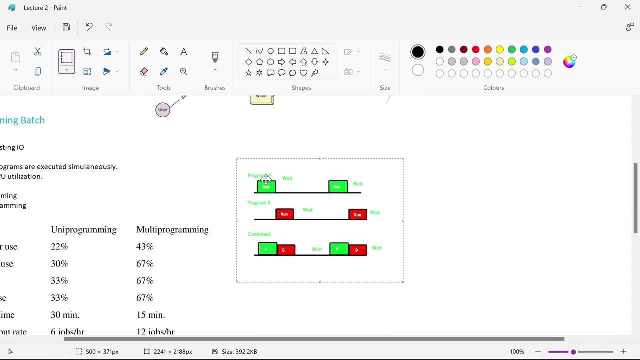 One second. So if you are converting that to multiprogramming, Then what we are doing, Whenever the processor, program A is not using the CPU, That means in the wait case, We can run program 2. You can see here this time: whatever we have now That we are assigning to the program 2, 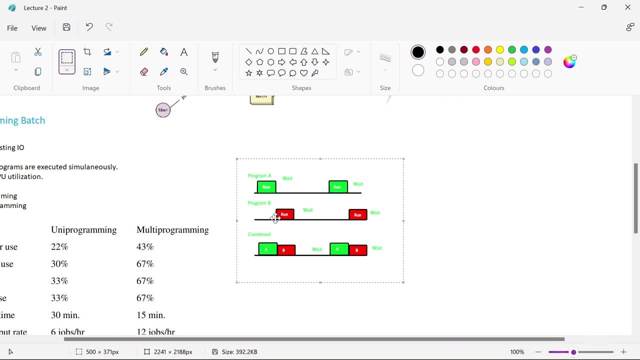 Got it Now. if it requires wait, Then also then it will be wait want you can have one more program where this wait time can be used. got it here. i have taken two programs only. you can have multiple programs, more than two can also be considered. but if you 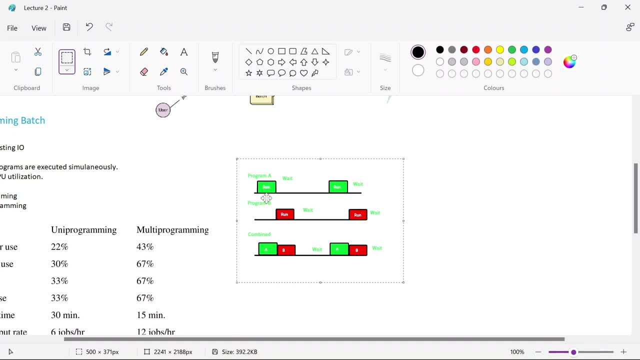 are using multiple. let us consider two programs. only if you are combining these two, did you see the wait time? that means the cpu wait time has been reduced or not earlier. in case of one program itself, the wait time is from here to here. we are wasting the cpu time this much, but if you are, 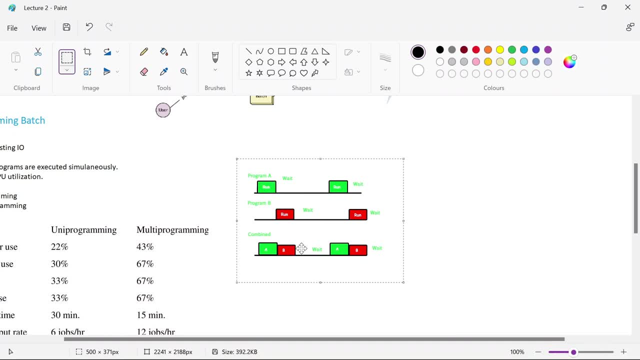 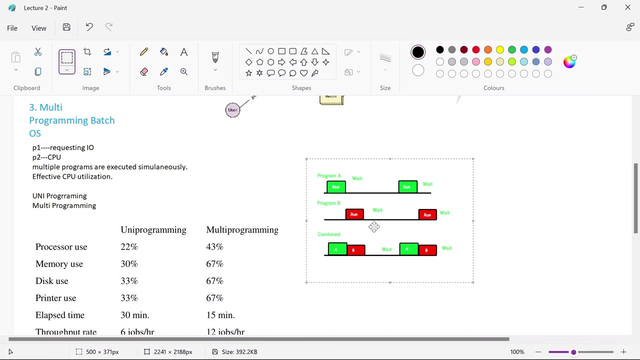 combining. as an example, i have considered two. only the cpu idle time is reduced or not. so this is what we are saying: 43 percent processor use is there and we are reducing the cpu wait time also here i have taken two examples. you can add one more program and this wait time can be used to. 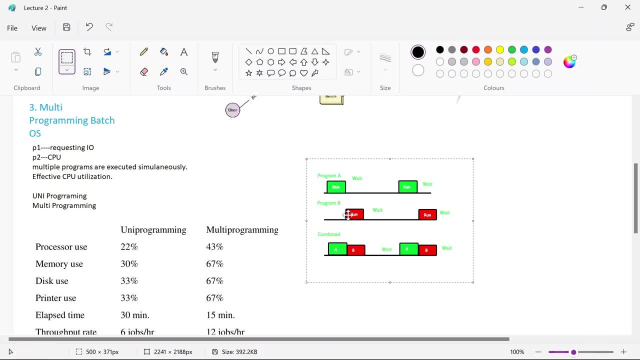 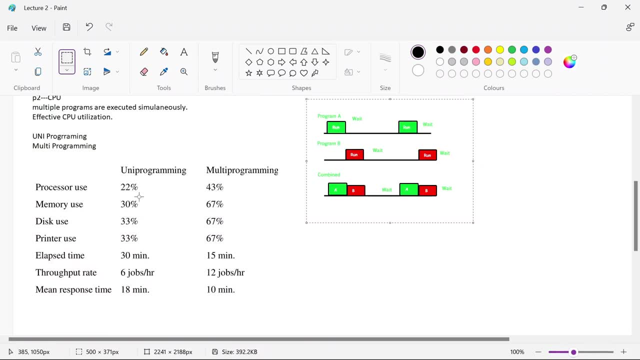 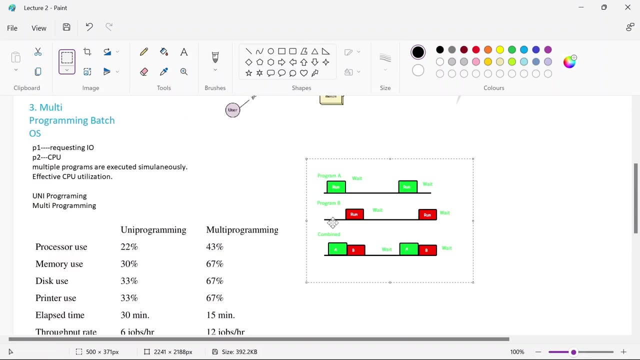 execute that program. okay, so if you keep on adding the programs, the wait time will be obviously reduced. and coming to the second option, that is, memory usage, 30 percent of memory will be used, whereas 67 percent of memory is used in case of multi-programming. why? because multiple. 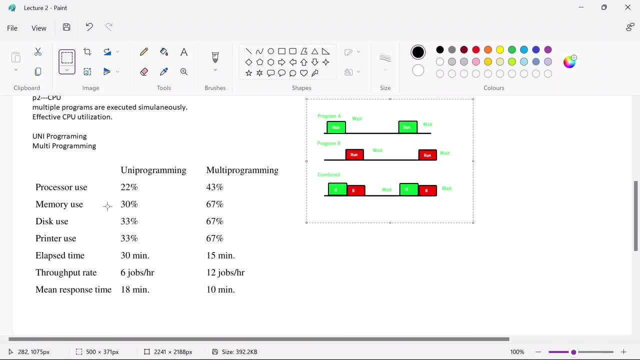 programs we want to execute simultaneously. all the programs should be available in the memory, okay. similarly, you can see the disk uses, printer use and elapsed time is 30 minutes. here it will be 15 minutes throughput rate, like how many jobs are executed, particularly for a particular time. 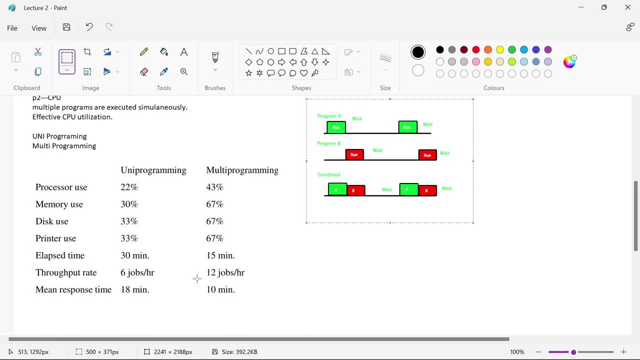 for one if for a particular hour, six jobs are executed here at the same time. we are doubling the number of jobs that are executed for a particular time for one if for a particular number of jobs that can be performed. that is 12 jobs here and the response time is 18 minutes, and 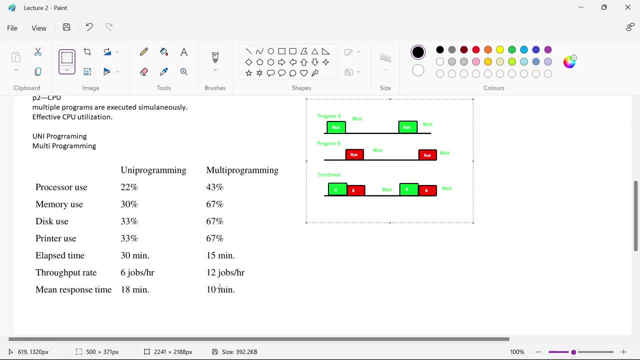 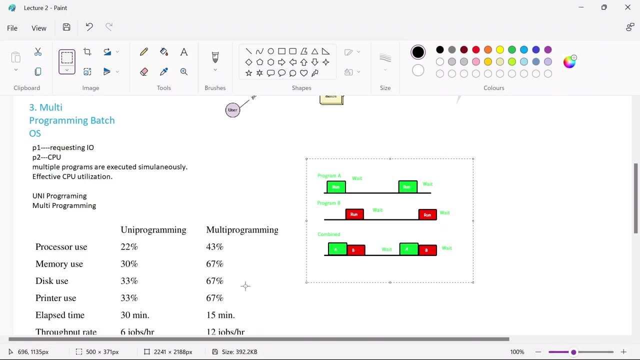 here. 10 minute time. response time is nothing but the amount of time required to finish that job. that includes the execution time plus your waiting time also got it. so this is about your multi-programming batch operating system. i hope you all are clear with this multi-programming. 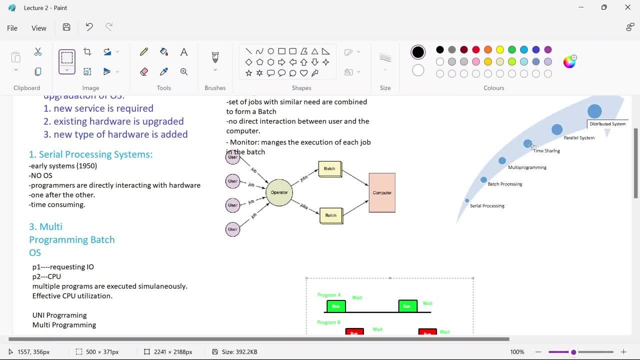 batch operating system. now we'll see the next category, that is, our time sharing operating system. that is a fourth category. keep your heading, all of you. what is the fourth category? time sharing operating system. now, what is this time sharing operating system in this time sharing operating system? 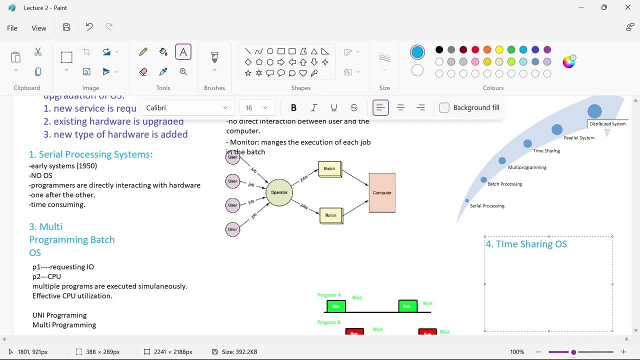 what happens is it is mostly similar, like your multi programming operating system only but the main. one more additional feature here is cpu will be allocating the time for all the processes. here there is no time. it is not like uniformly. we are allocating the time for all the process. program a how much time it want to execute. it can execute if. 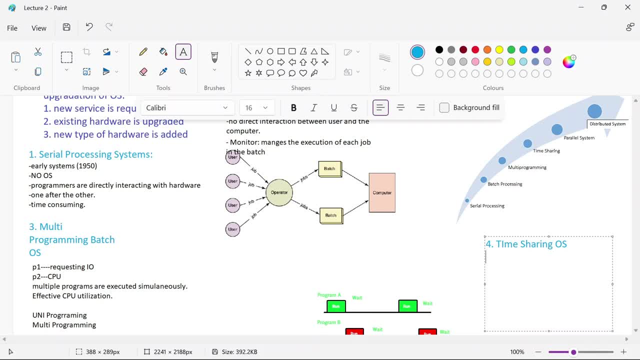 any weight is there, then only it will be switched to the program b. but whereas coming to the time sharing operating system, what happens is cpu time will be allocated. the cpu will be allocating time for the programmic RJ-700 project. allright, once again, timesharing ofthis Hlerin videos up to the 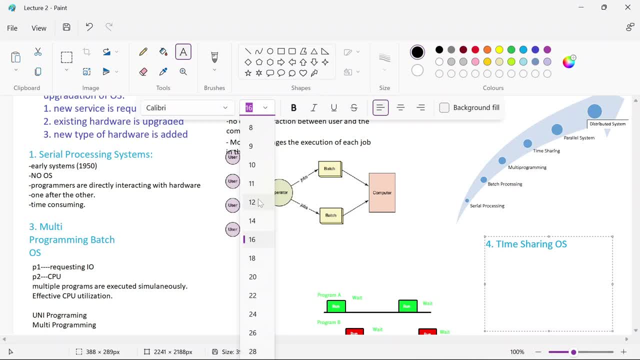 forthإ the future which can have more upload rate and cost infinity plus- this is what they used to do- multiple process. that means we can assign some time for each and every process so that, even if it is not going for a wait, it can be forced here and it can be executed okay. so we can understand. 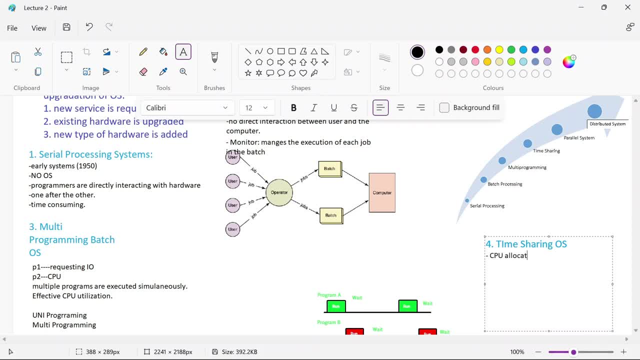 here cpu allocates time for each process, and rest of the things are same, like your multi-programming batch operating system. only the only additional thing here is cpu allocates time for each process that for that much of time it will be executing that one. so this also is used to reduce the cpu. 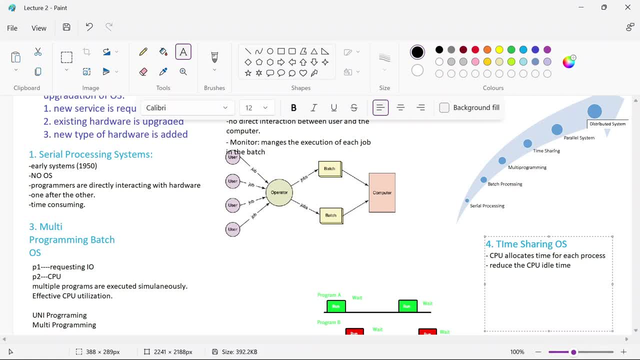 ideal time. okay, so the only one extended feature is there, when compared to the multi-programming in the for the time sharing operating system, that is, it allocates the time for each process. okay, here also, the response time will be less. i think you all understood what is response time. 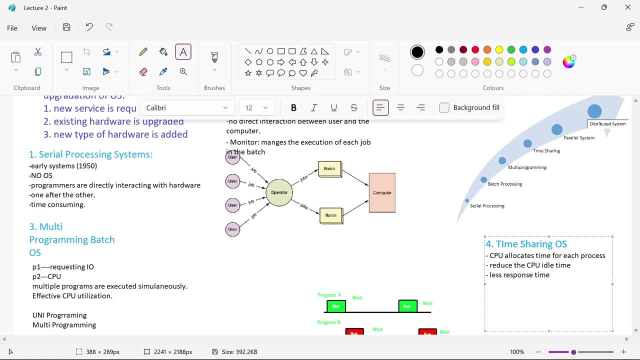 response time is a thing, but time, in simple words, if you want me to tell you like the amount, the time between the input and output is called as a response time. okay, if, once you give the input, you are, you are waiting for your output to be generated. so the time between the input and output is called. 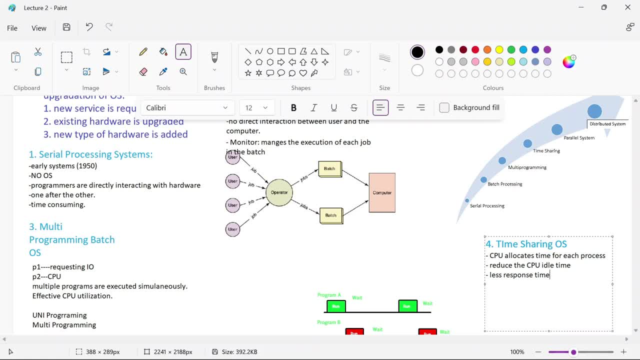 as a response time. so in time sharing operating system also we have a less response time. that means we will get the response quickly and the ideal time is also very less got. it is that clear. so understand here. serial processing operating system- it has come in 1950- and multi-programming um. the second category, that is batch programming. 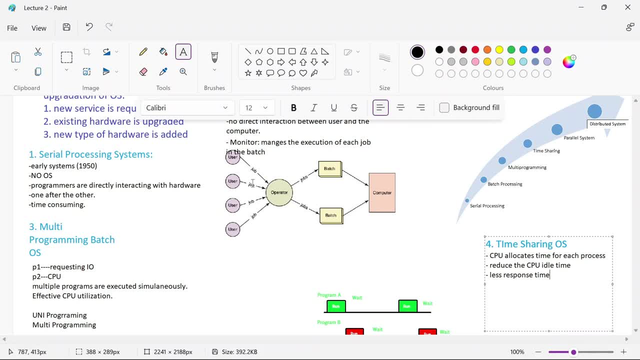 system that is gone, that is evolved in 1960. this one in 1960 that is multi-programming batch system, is in 1960 and this one multi-programming batch operating system. this is in 1970. i'll just make a note here. 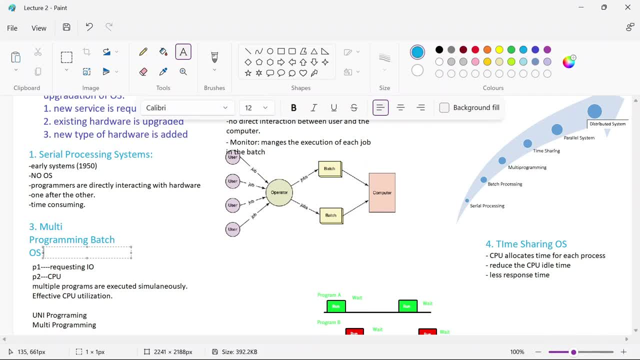 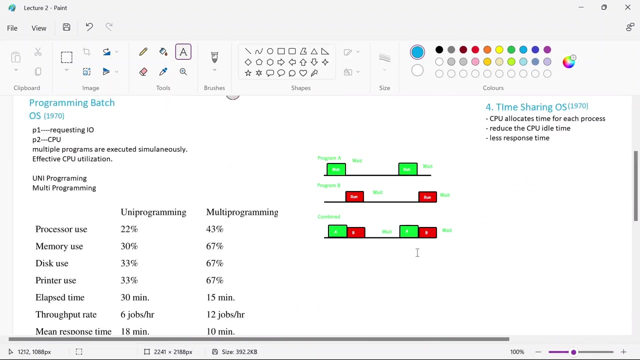 so that you can note down 1970 and time sharing operating system, also in 1970. okay, i hope you all are following this one. okay, now let us move to the next type of operating system, that is, parallel systems. that is our fifth category. keep adding all of you: parallel systems. 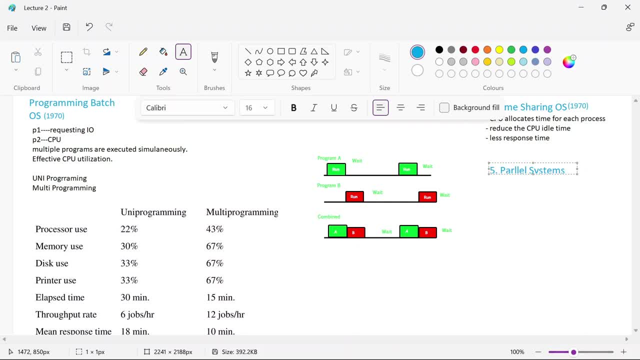 now, what is this? the new category? what is the parallel system? parallel system is nothing, but we will be having here more than one cpu. as of now we are considering, as we will be having only one cpu, but in parallel systems. what we are considering is we will be having more than one cpu. okay, more than one cpu is more than one. 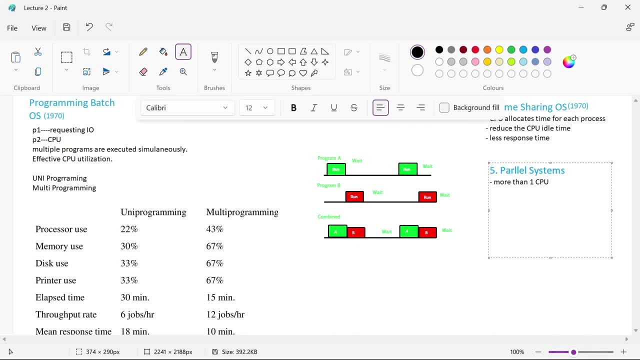 processor. that means multiple processors. whatever we have now, they have directed to share the memory. in this we have multiple processors, all the processors. all the processors are sharing the memory, whatever is available. so as all the processors sharing the memory, they are called as tightly coupled. i'll show you how to do this. 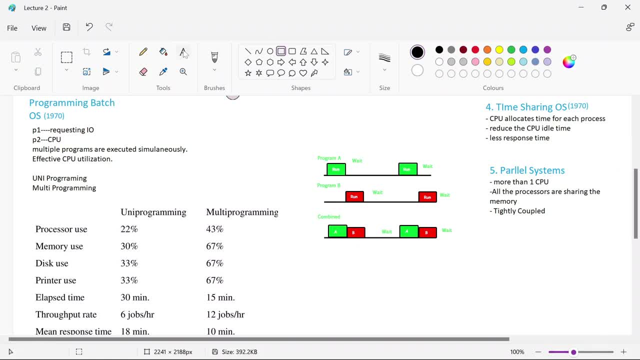 i'll show you how to do this. i'll show you one example here. you can see, let us consider, this is one cpu. okay, so as we are considering, we'll be have, we can have multiple cpus we can consider. let us consider as an example. i'll consider: 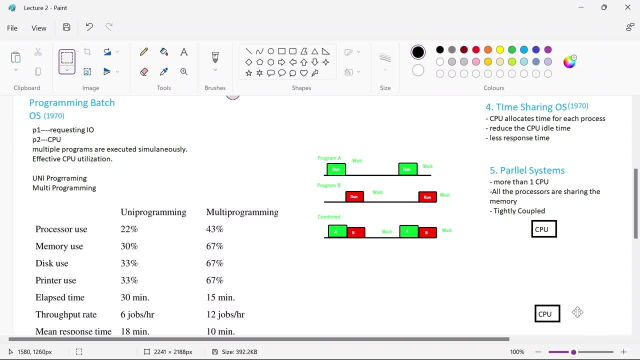 four cpu: cpu1, cpu2, cpu3, cpu4, cpu5, cpu6, cpu7, cpu8, cpu9, cpu10, cpu11, cpu12, cpu12, cpu13, cpu14, cpu14, cpu14. let me consider the third cpu and one more cpu, fourth cpu now in a system see: 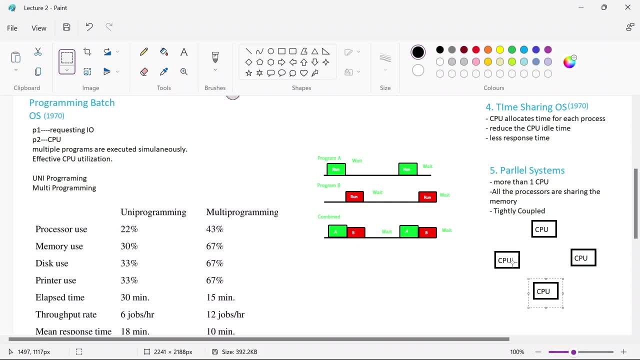 this is not the case, like in one system, always we should have multiple cpus. that may not be case. we can have multiple systems also. all the systems are connected together. but make a note, here it's all the CPUs should connect to a single memory, like only one memory is there and all the CPUs. 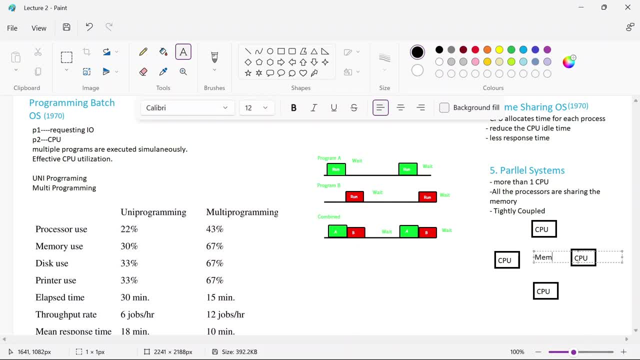 are using that. So now what you can understand, this CPU is using this memory and the same CPU will be used by this and the same memory will be used by this CPU. this CPU will be using this memory and this CPU will be using this memory. 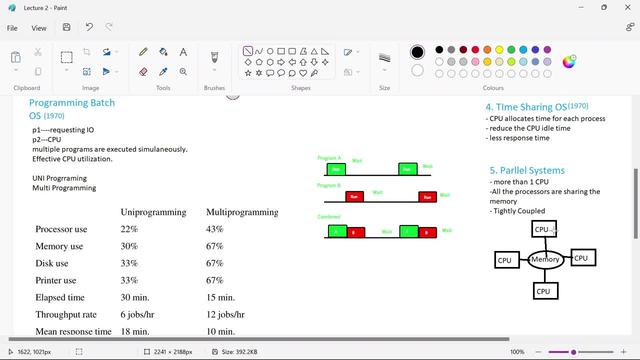 Okay, so this is called as parallel system. Now, what is the use of having multiple CPUs? is here: it is used to speed up the execution of the program, like if a single problem is given or a single process is given, two or more processes or two or more CPUs work together. 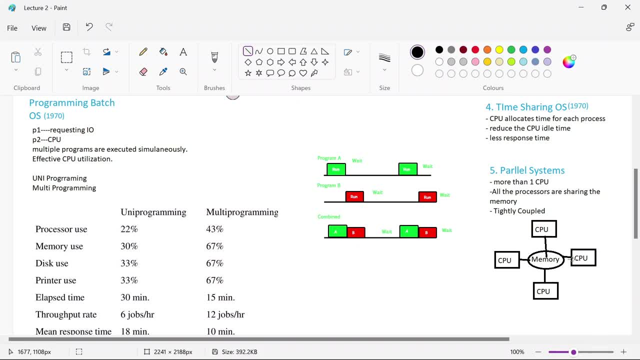 they can combinely, work together to get the solution for that problem. that is what that is here. we want to speed up the execution time, we want to reduce the execution time. that is the main task of having a main Reason of having more than one CPU. but the main observation here is you need to have 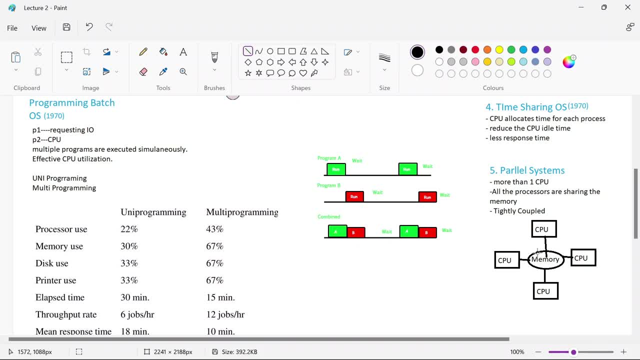 like all the CPUs are using the or sharing the common memory. okay, it will be. it will be doing multiple things at the same time. So you can say: here it is time saving and it will speed up the execution of the time, and it will be doing multiple things at the. 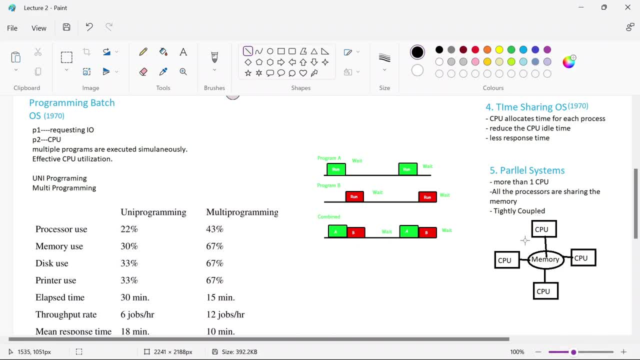 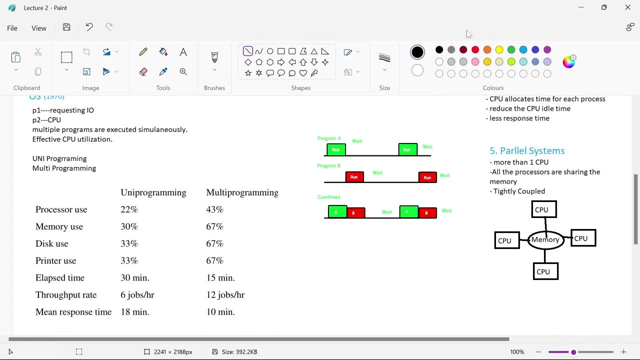 same time. that is what parallel systems is okay. Now let us go to the next type. what is that? distributed systems. So keep adding all of you. Second, sixth category is distributed systems. Distributed system, operating system, is nothing but Understand here. 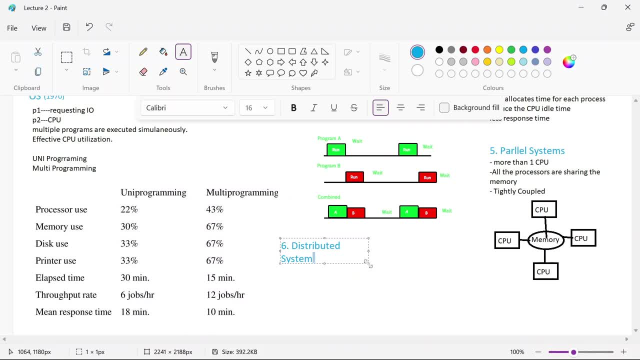 in parallel operating system. same like your, this one parallel operating system. here also we will have more than one cpu. but the difference between the parallel and distributed is see here also more than one cpu, here also more than one cpu. and both the in both the cases our main motto is to get a. 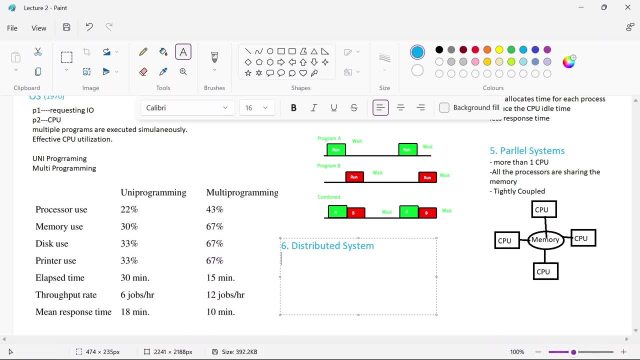 solution to a problem more quickly. all the cpus will be communicating together, like all the cpus will be combinedly used to get a solution for a single problem. got it now here. what? in the parallel systems the memory will be shared, but whereas in the distributed system memory will not be shared. 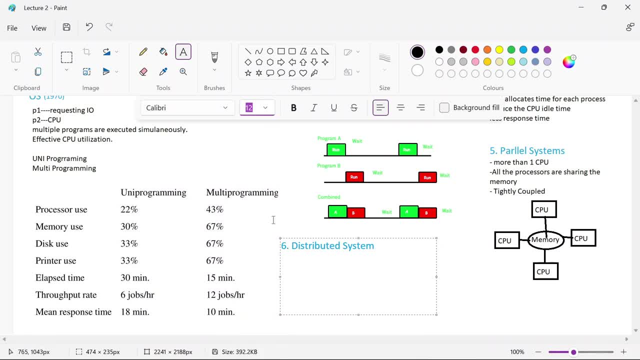 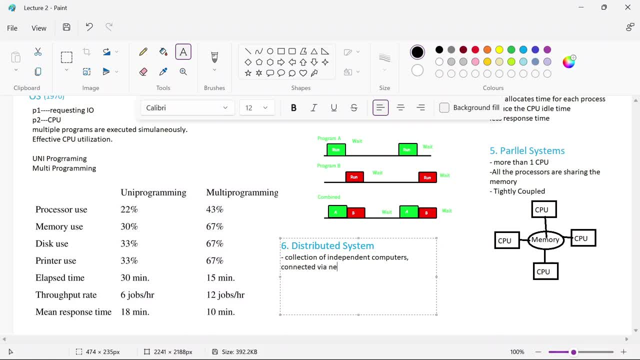 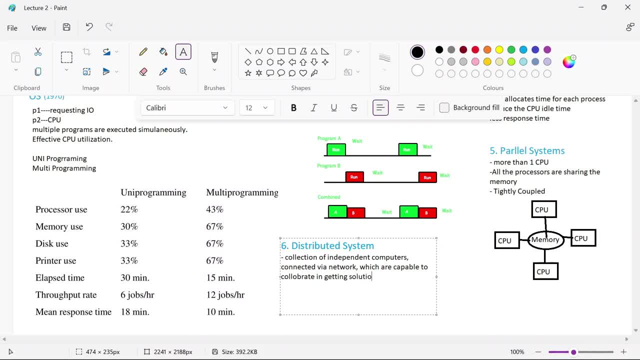 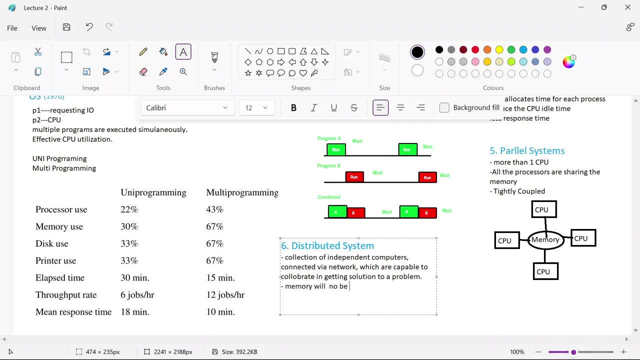 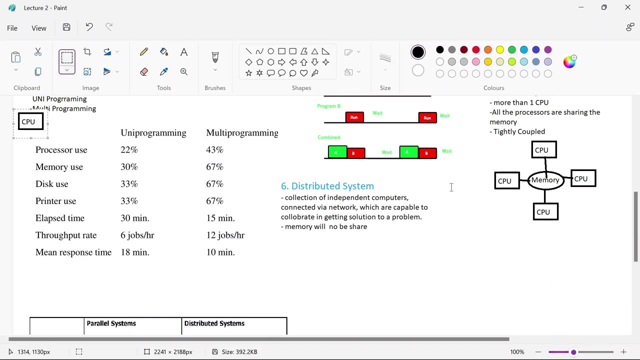 be shared. that means we will take one example. I will draw the diagram here so that it will be clear to you. CPU will be there and then memory will be there. okay, and this is combinedly called as one system. each system has its own CPU and its own memory system. 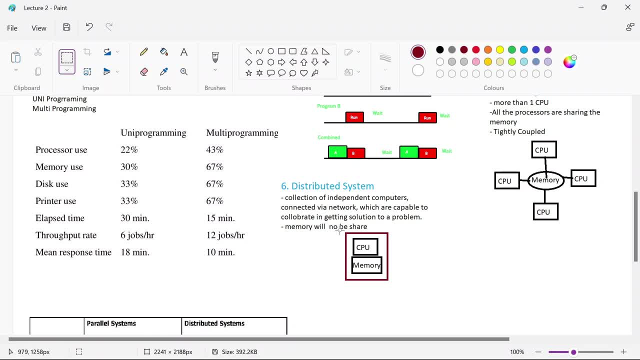 I hope you all are following. this is one system. now, like this, we can have multiple systems. let us consider: this is system two, and let us take one more system. this is system three, and let us take one more system. that is system four. okay, now all these systems. 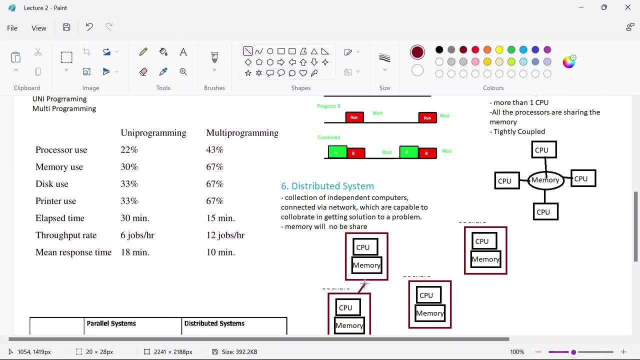 are communicating. all these systems are interconnected together with each other, where they will be communicated through or connected through the system, through a network, and they will be passing the information among themselves. and all these will be communicating together. why? because they want to get a solution to a 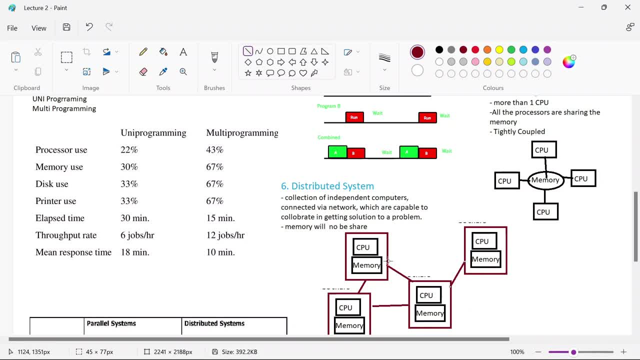 given problem. they will be collaborating, which are capable to collaborate, and they will be giving the solution to a problem. so these are all independent systems. observe the difference between these two. we have CPUs and the memory shared in case of parallel systems and the distributed systems, each system. 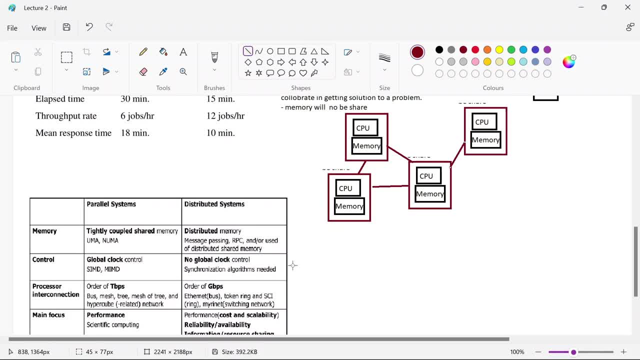 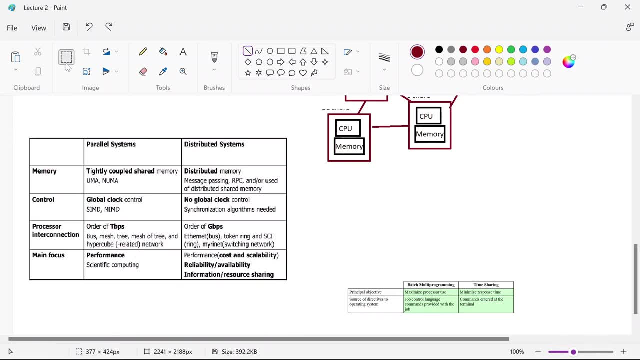 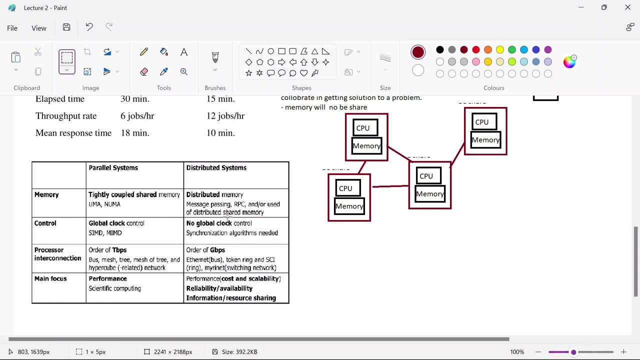 have its own memory other than this. here I want to highlight some of the differences between the parallel systems and the distributed systems. just go through this all of you. in case of memory- it is already told I have highlighted here- the memory is tightly coupled. why? because the memory. 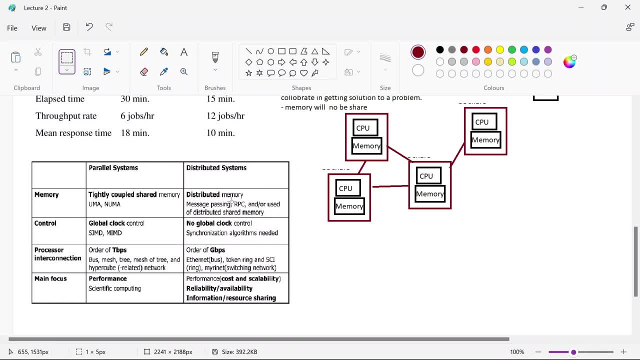 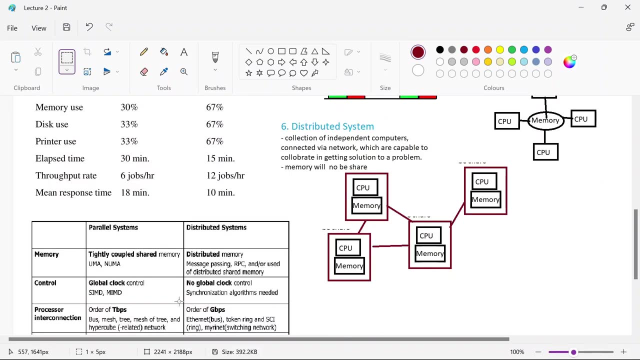 is shared in case of parallel system, whereas in distributed system it is loosely coupled. ok, and here in parallel system, we will be having a common clock. ok, in parallel system there will be a clock that is commonly used by all the CPUs- ok. but whereas in case of 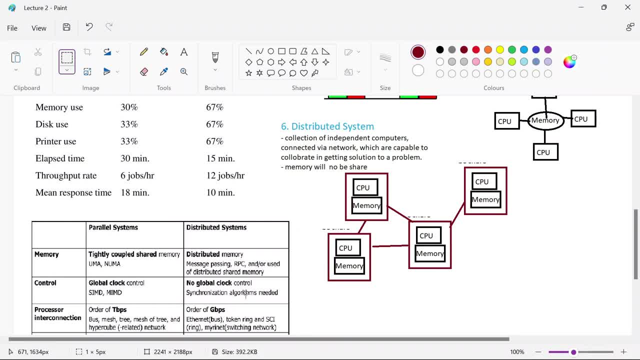 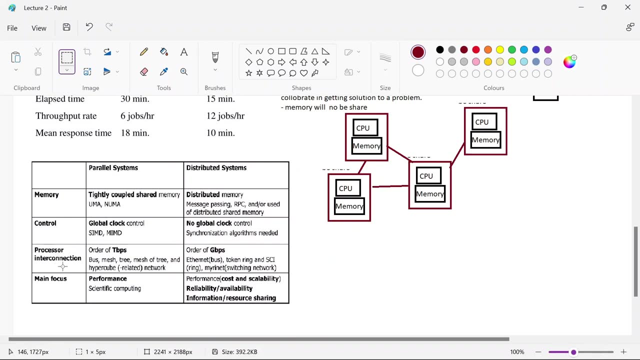 distributed system there is no global clock. some synchronization algorithms are needed here. so here clock is there to make them synchronous, but whereas in distributed system there is no global clock control, some algorithms are required here. ok, and here the processor interconnection will be in the form of: 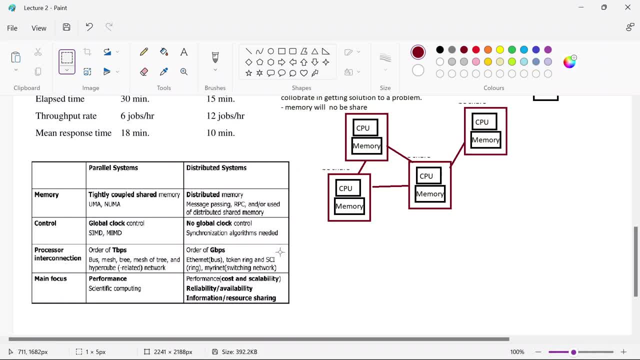 TPPS, whereas in the here distributed system it is in the order of GBPS. ok, so they are connected through the network. it can be an ethernet- one example can be ethernet- whereas, coming to parallel systems, they are connected together in the bus form, using bus connection or 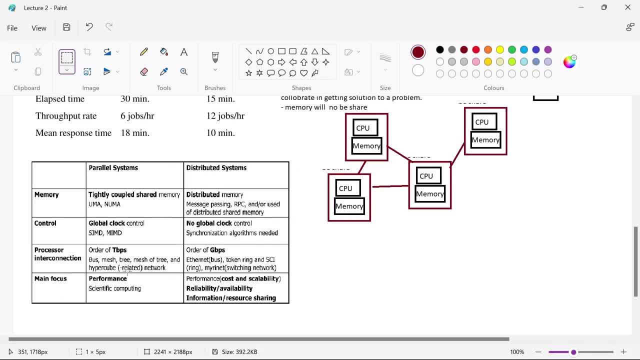 mesh or tree form like that. the main focus in the parallel system is to performance. ok, and it will be mainly used for scientific computing, only where the memory will be shared. but whereas in the distributed systems what happens? is it the same, like performance also, and reliability, and 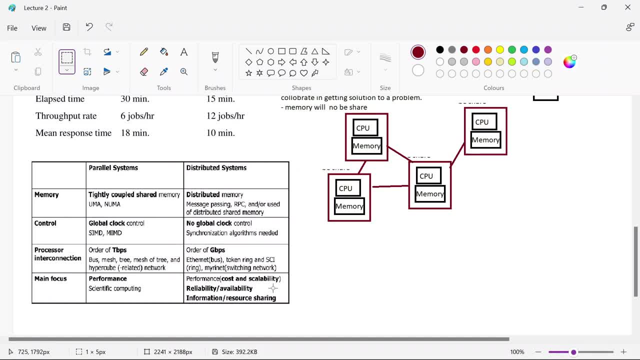 information sharing and resource sharing. if you want to do, then also we can go with the distributed systems. ok, one example here is, like you can see: ATM machine, that is an example of your distributed systems. telephone network, that is an example of your distributed systems. ok, so this: 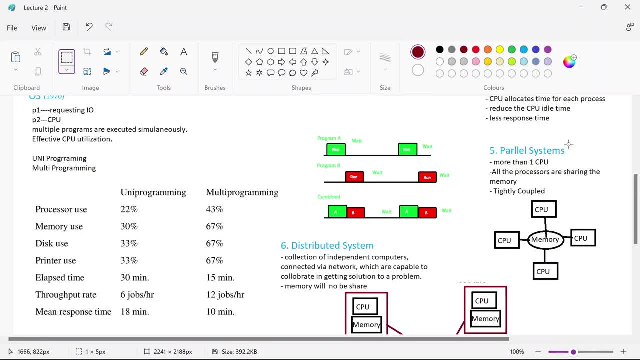 is also has come in 19, I think, 1980. parallel systems and distributed systems has come, so make a note of that one out of you. this is in 1980, ok, and distributed systems are also in 1980, ok. now coming to the next. 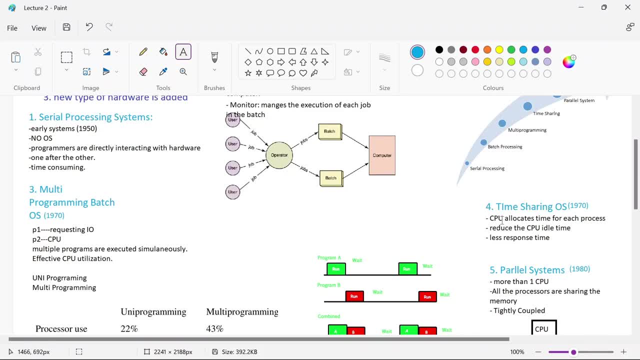 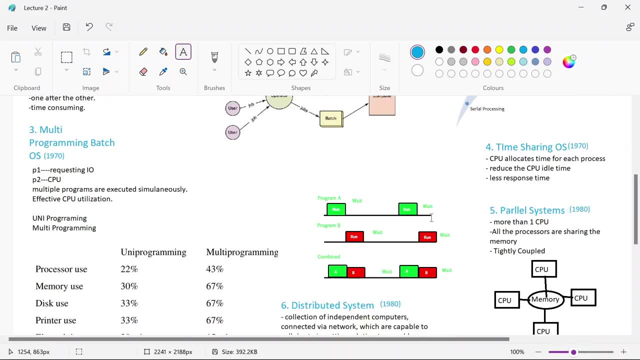 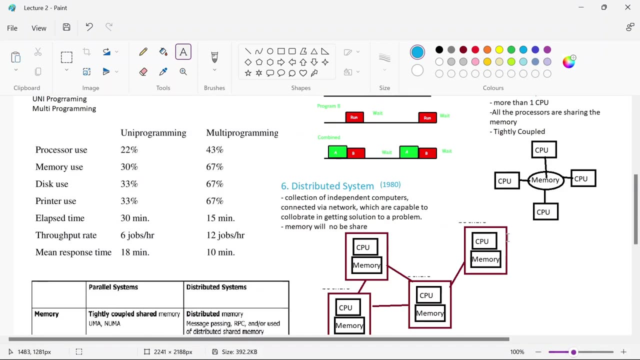 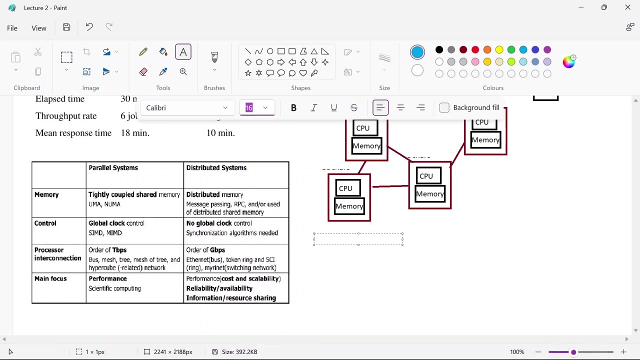 category. this, like we have the two more categories, like two more types of operating system, that is about personal computing systems and real time systems. let us quickly go through that so that we can. so this is of 7th type. ok, now what is this? personal computing? 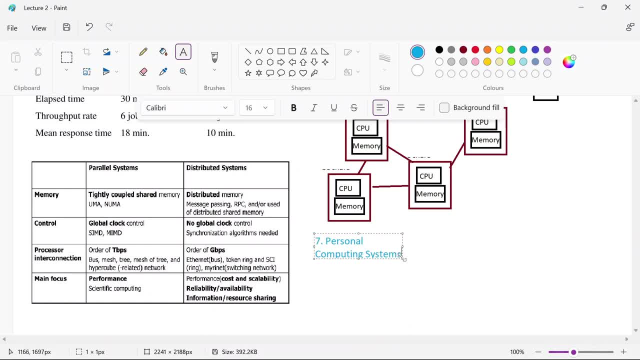 system is personal computer, as the name itself it is reflecting. here, personal computing system is nothing but a device or any gadget. if it is used by a single person, then it is called as a personal computing systems. ok, not done all of you. so that means single user. 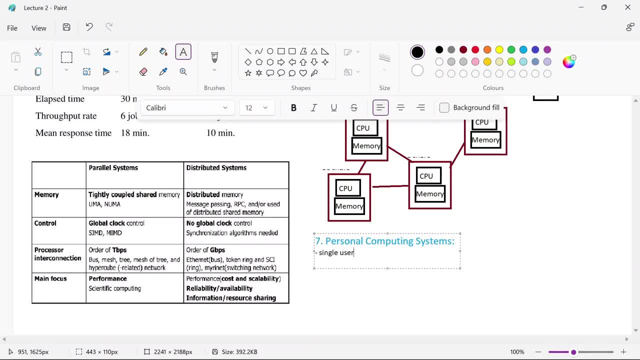 single user will be there. now what is the requirement of having such type of computers and an operating system within that? one is to have a portability, got it. so there are like the main reason here is portable and user convenience, got it. so that is the main. 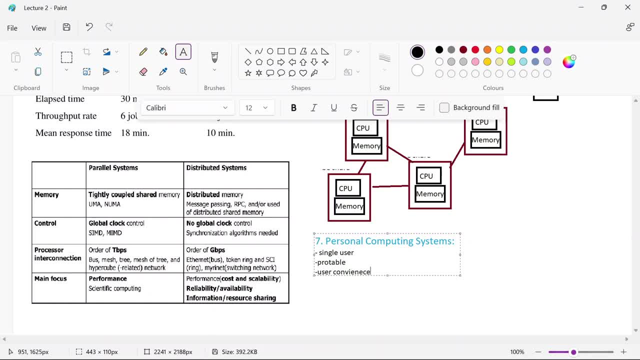 advantage in this also, like if you don't want to have an advanced cpu utilization, then you can go with the personal computing systems. so in these systems, these systems may not need, or they may not require advanced cpu utilization. then such things are called examples. you can make a. 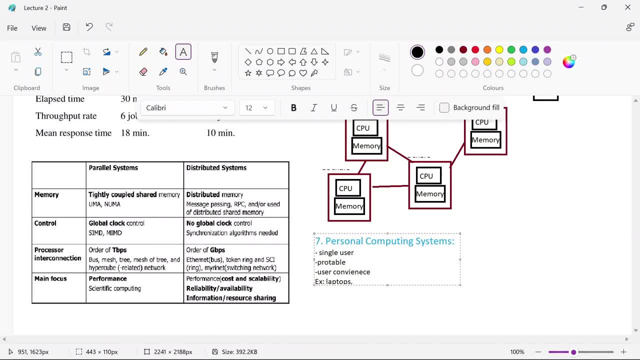 note of this one. your laptops. you can use desktop. all these are used by single user and laptops are very portable and user convenience also. i hope you all are clear with this seventh category, that is, personal computing system. this has come in the year nineteen, eighty, okay, and the 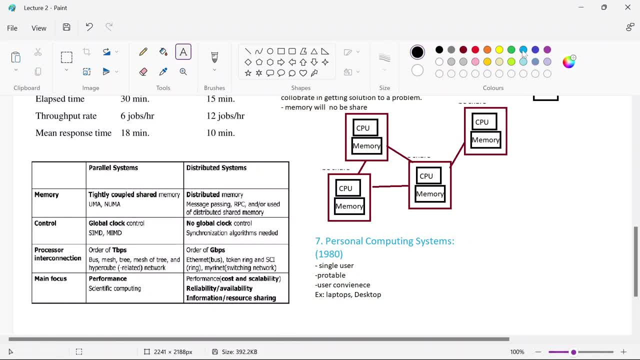 last type of operating system is real time operating systems. eighth category: not done all of you? now, what is this real time operating system is? these are mainly used to implement the real time applications. one example i want to highlight here is what is nothing but real time applications. 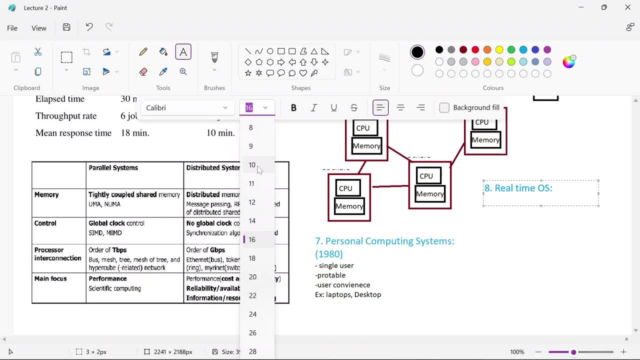 let us consider an example of designing a driverless car. so in that case, we need- that is a real time application, isn't it, or not? so it has to respond immediately. now these systems. let me note down first that one: these are used to implement real time. 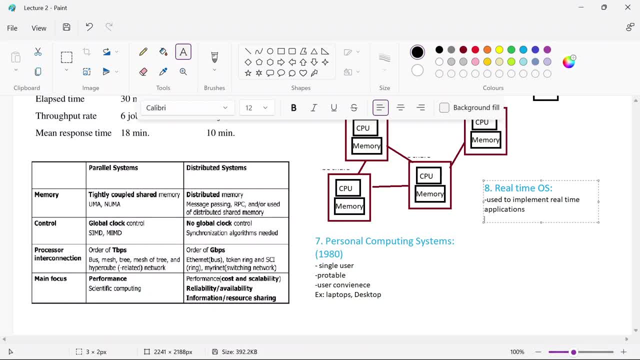 applications. now what is the main requirement of having this one is it has to respond immediately when an input is given. that means when an input is given, response to input immediately and produces output. so i will take one example here. let us consider a driverless car. is 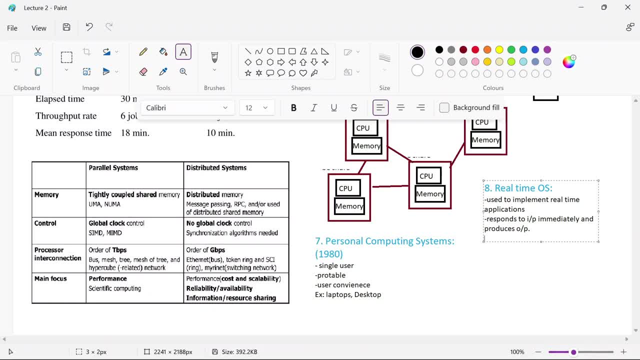 there then the in that car, which is completely automated. now there are sensors connected to that one. now, whenever anything comes in front of that car during the driving process, then it has to quickly recognize that input, like some obstacle, is there in front of that one, and it has to put the brake and stop that car that way. 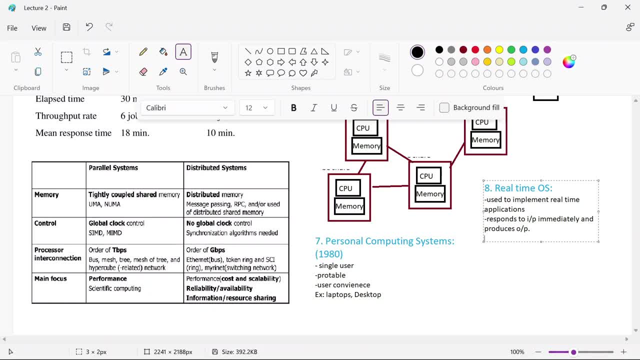 that means for an input, it has to immediately respond and produce and generate the output. that is what this is. an example of real time operating system: ok, such operating systems are there. two types of real time operating systems are there. first one is ok. first category is which is: 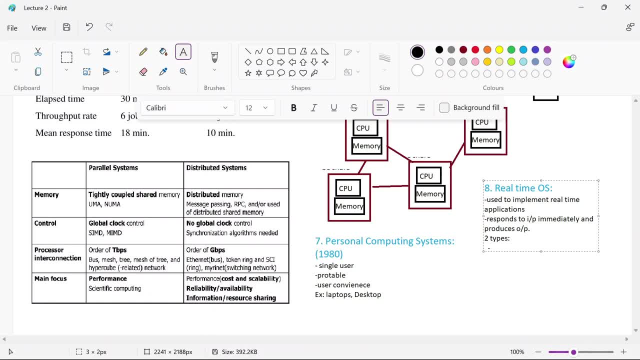 called as hard real time operating systems RTOS. what is called as hard real time operating systems RTOS, what is called as hard real time operating system, is the application. like there will be a stipulated amount of time. within that time only, it has to respond or it has to be executed. 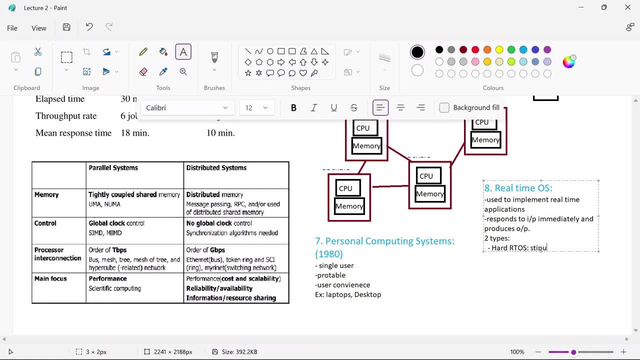 ok, in a given time or in a stipulated time, it has to be. it has to finish the execution. the same example you can consider. that means immediately. once there is an obstacle is observed immediately, within a fraction of seconds, it has to finish the execution and act accordingly. 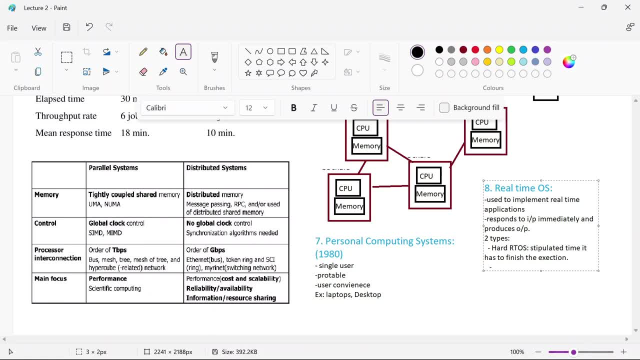 ok, that is an example for that one, whereas we have another type, which is called as soft real time operating system, where it is ok, even if you are not finishing. or if you are not finishing the execution in a stipulated time, then also it is ok. such a real time operating system is called as: 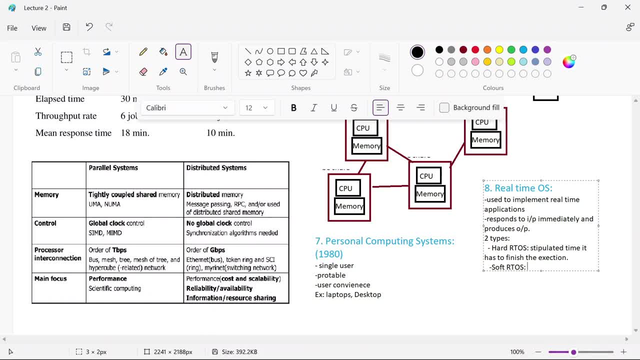 soft real time operating system. it is not like all the real time applications need to have the feature of immediately finishing the execution time in the stipulated time. it is not like always it should be hard. real time operating system: it is ok even if you have not executed.